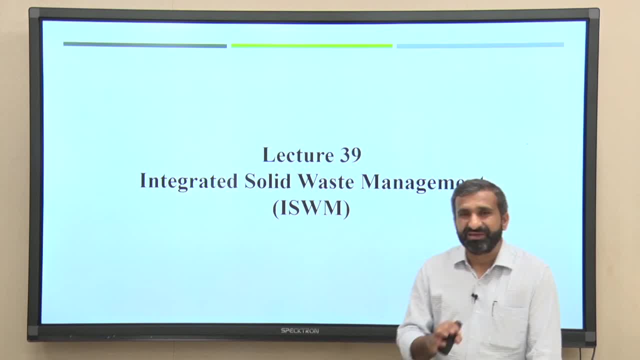 as an integrated solid waste management plan. But it is not true the. that is why I thought of to have one special discussion on to the integrated solid waste solid waste management plan or system And also need to know that how the one local corporation or local authority or ULB will. 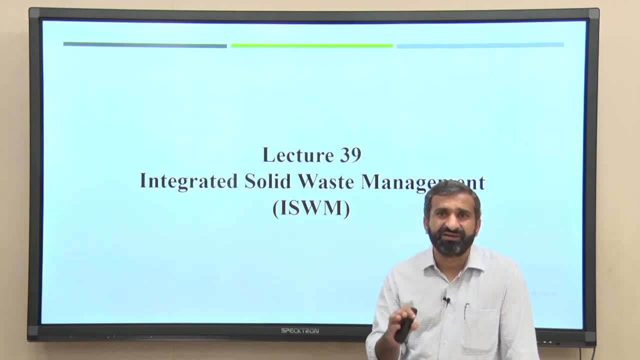 prepare the plan. This plan is specially is explained in the manual- solid waste manual at 2016.. So I thought of the. this should be known to the students also how the corporations are normally planning the entire solid waste management plan. So first we will start from. 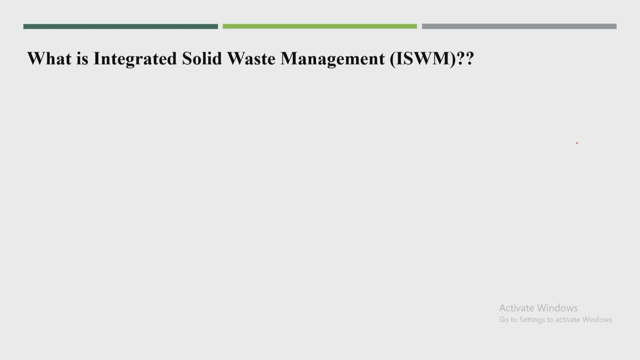 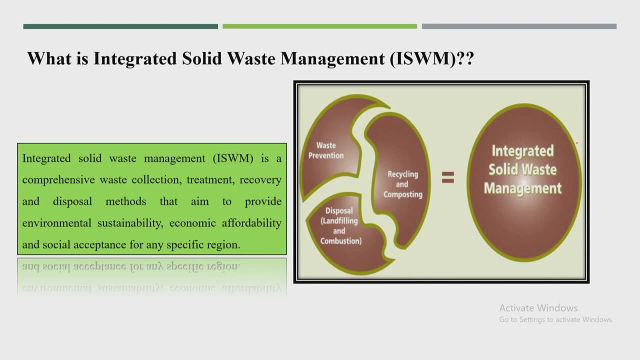 the integrated solid waste management plan. So first we will start from the integrated solid waste management. So first, what is the meaning of integrated solid waste management is a comprehensive waste collection, treatment, recovery and disposal method that aim to provide the environmental sustainability, economic proper and special social acceptance from 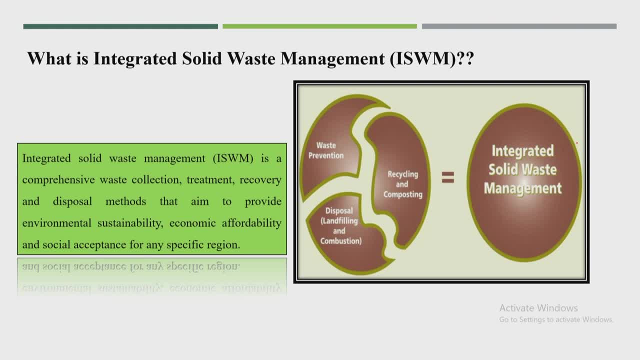 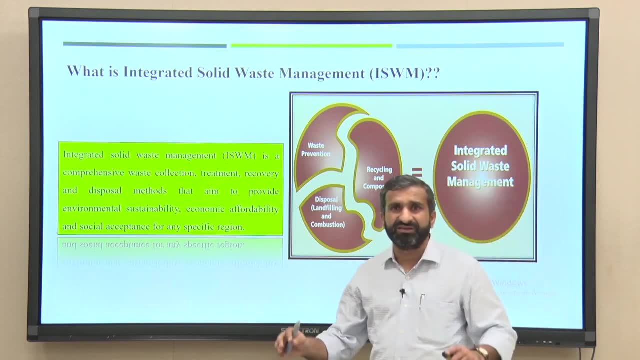 the specific region. So this is the few important idea about integrated solid waste management is a. it is including all physical elements of municipal solid waste management based on the environmental sustainability, the economic way and finally, it should be accepted by the local areas, socially also should be accepted. So this is called integrated solid. 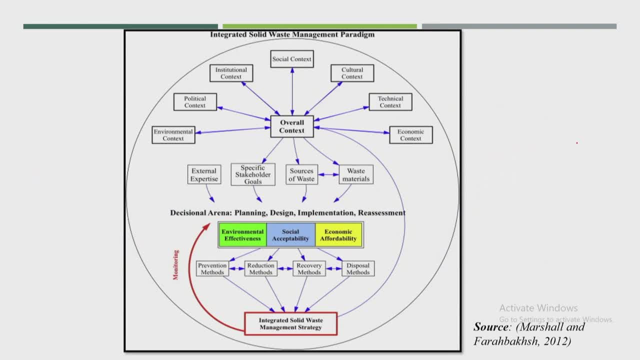 waste management system. So when you say the idea of what integrated solid waste management strategy, So once you have something like a this, you know sort of what you expect: how you get out of this, How you get that out of the tractor or just getting the s? 죽. So first, how? 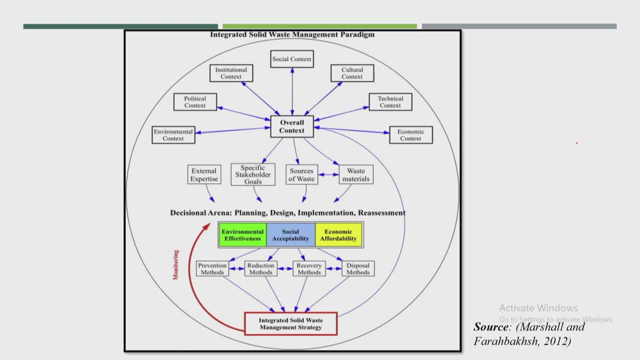 you then use the s, integriate treatment and76 other things like sodium. it would be somehow the major piece of all elements, and it should also be an area such that the region that〜you have 해� So, which is including the entire issues about the solid waste management system, like it. 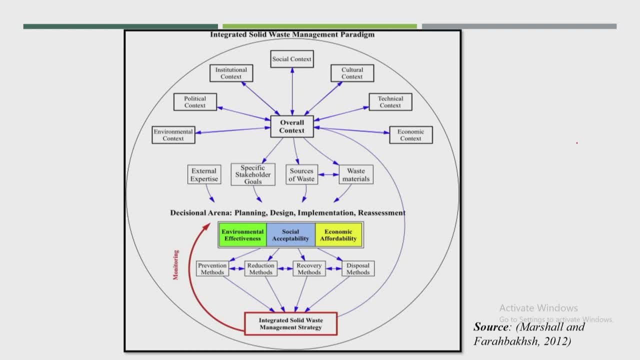 is starting from the culture, culture, technical, economic, these all, all the social as well as economical, technical context, and after that it is also including the waste material: what kind of sources, different stack holder and finally it will go to the planning or 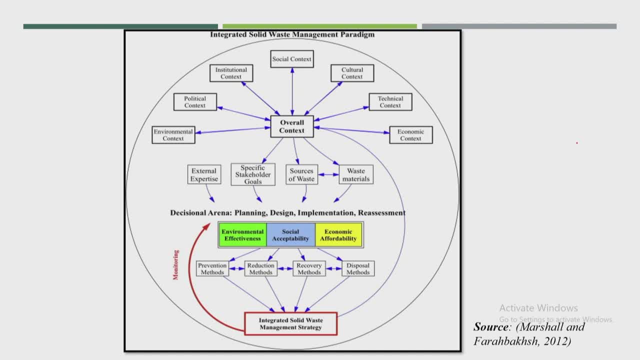 designing or implementation of integrated solid waste management plan, And that has to be also except on the three basis, like environmental, social and economic constraint has to be except And based on that, how best we can prevent the waste, reduce the waste, recover or how. 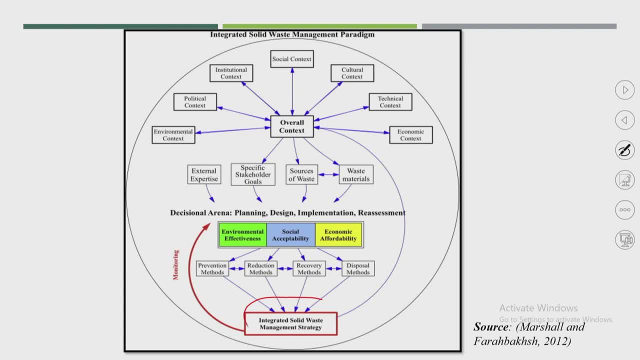 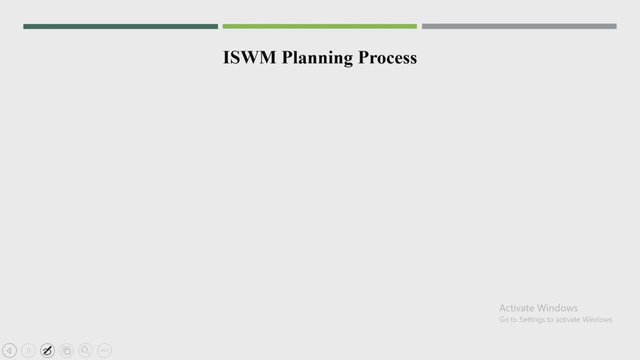 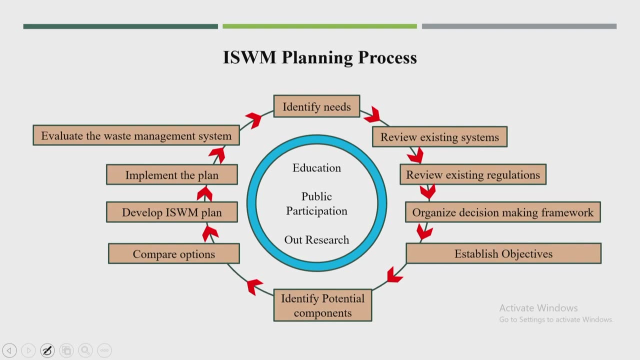 best we can dispose the waste. that normally called as a integrated solid waste strategy. So what is the ISWM or integrated solid waste management planning process? Normally it will start from the identify need need first you identify, review the existing system. Review the existing system. 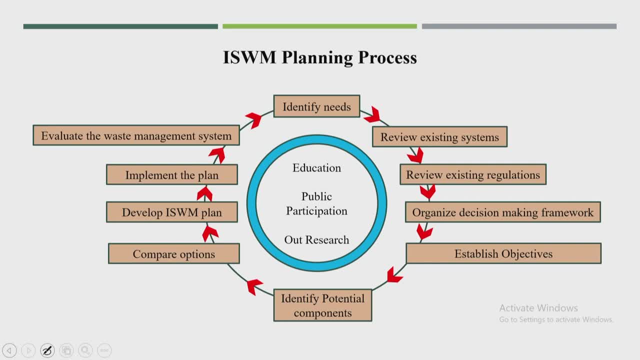 Existing regulations, what are the available in the particular region, a particular city or particular state, and then organize the decision making framework by calling the different stack holders and then, finally, you establish the objective. Okay, so once the objective is finalized, then try to identify the potential component. 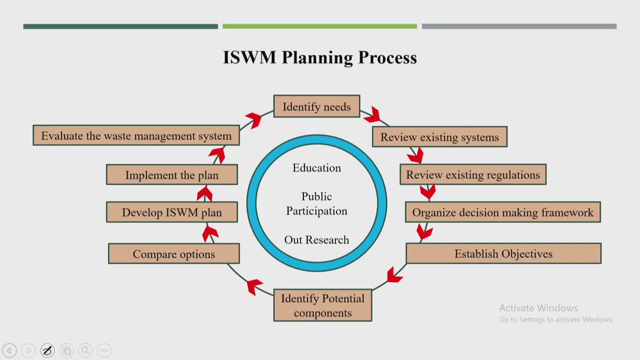 like was the objective will come up, like we can go for treatment process, Like biological treatment or chemical treatment, kind of processes that then see that the potential component of that, then compare the option, what are the different options, and based on that you develop the integrated solid waste management plan. and once the plan is ready, 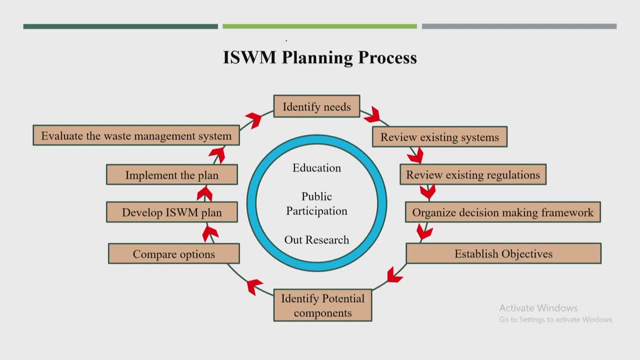 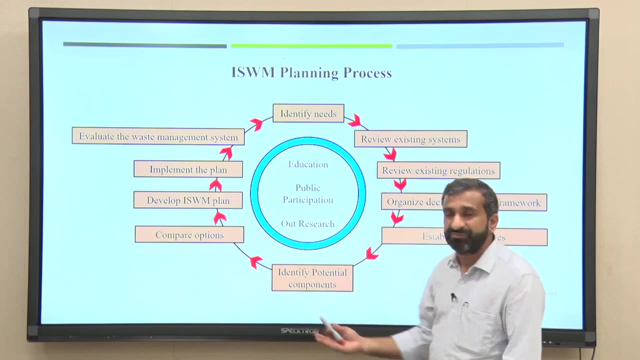 then try to implement how best we can implement that and then evaluate the complete waste management system. So likewise Again. So you can go by, you suppose. if you are not benefiting the particular objective or is not possible to achieve, then again go go in the same way. 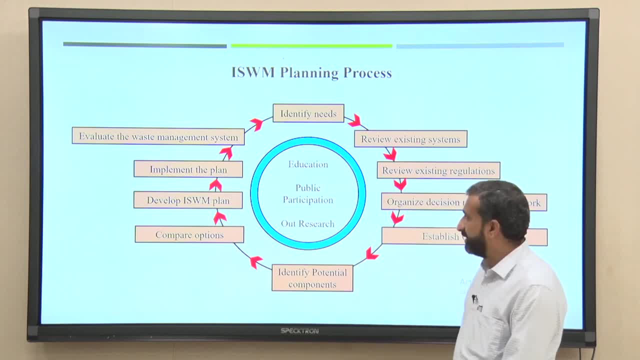 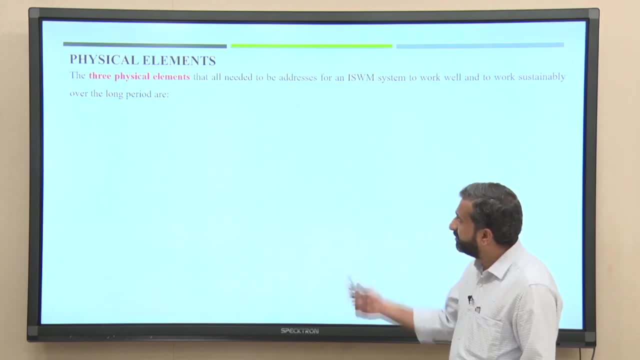 So likewise we can go for integrated solid waste planning. Now, when you say the integrated solid waste management plan or system or strategy, normally we will talk about the three physical elements and three governance features. So there are six features or elements are need to be discussed under the integrated 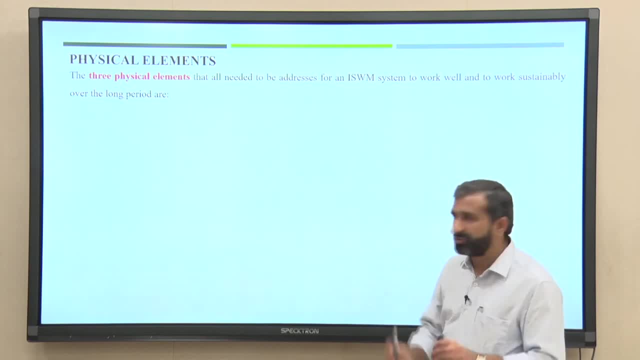 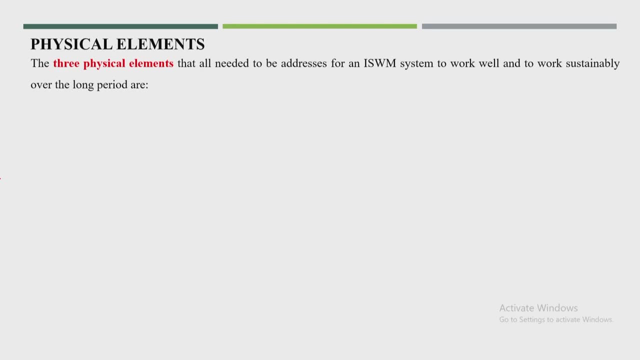 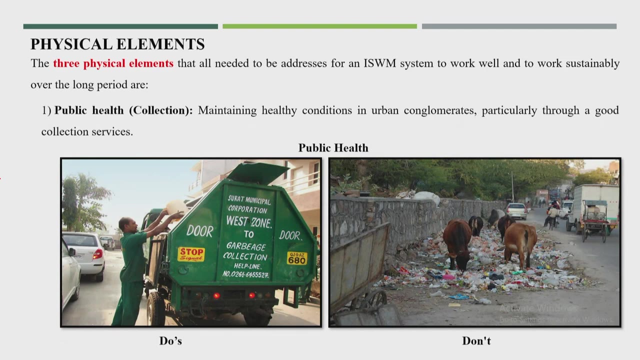 solid waste management plan, strategy or process. So the first. we will start with the physical elements, So the. there are three physical elements that need to be addressed. The first is the public health. So now the. what is the benefit of ISWM? 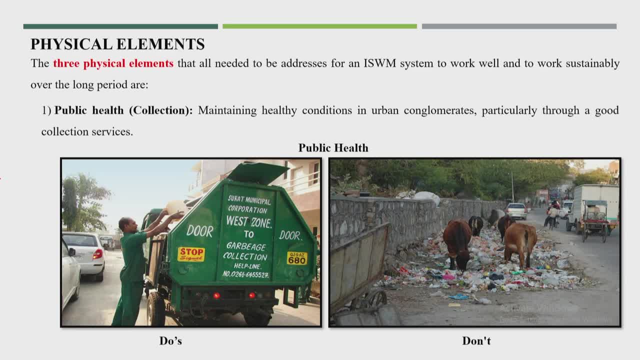 Is that Normally we called as a collection, by by proper collection. So rather than collection, why not to call as in public health? So the objective could be how best we can see the public health of the local people, So how the we can maintain the public health properly, the by maintaining the healthy condition. 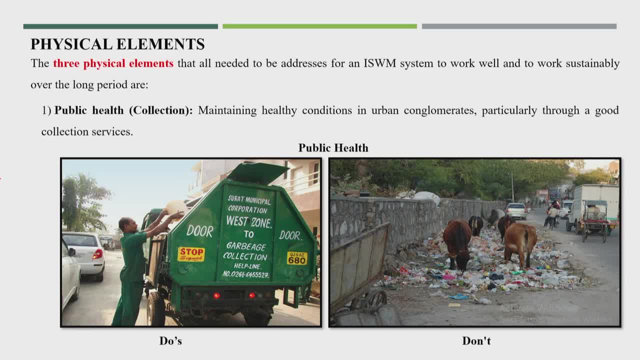 in the urban, urban location, particularly through a good collection services. So suppose these kind of collection system, Like how stores collection systems are available, like as it is start in the Swachh Bharat Mission, that that is the best kind of primary collection and secondary collection could be possible. 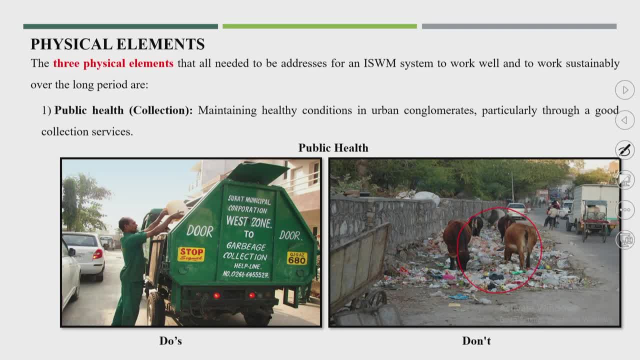 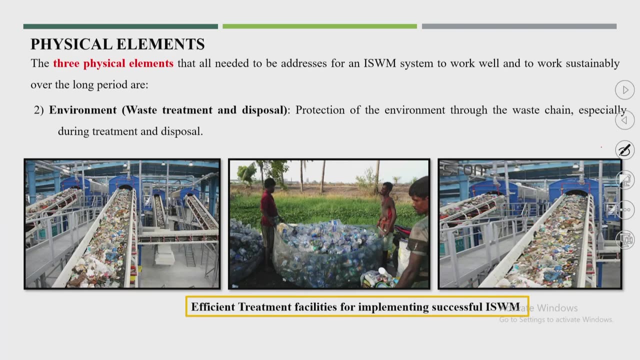 But if you have the this kind of collection or storage, I think it is not good actually, And because of that, a lot of public health issues will come up. Next is the environment. So now, how best? Now, how best, How best. 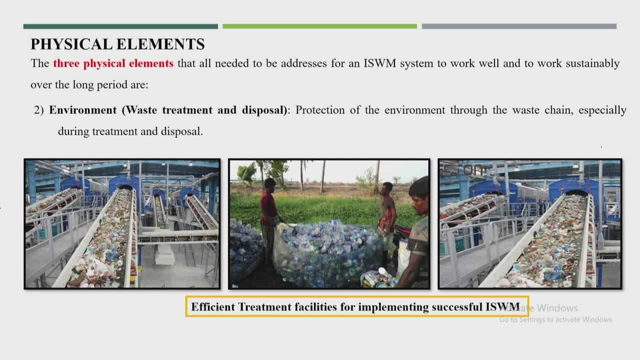 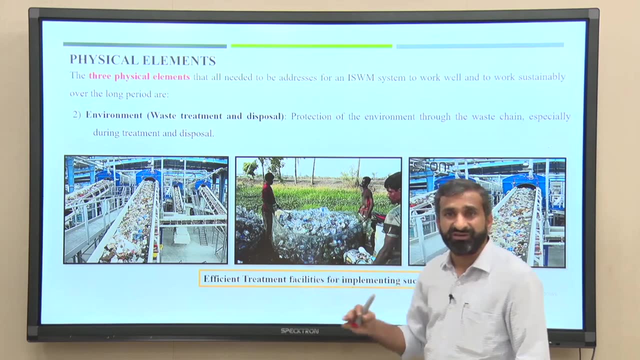 We can maintain the environment. So this environmental condition will be maintained, especially by waste management and waste treatment and disposal. If you are able to treat properly all kind of collected waste and also the proper disposal of entire waste, then then is good for the environmental conditions in the local area. 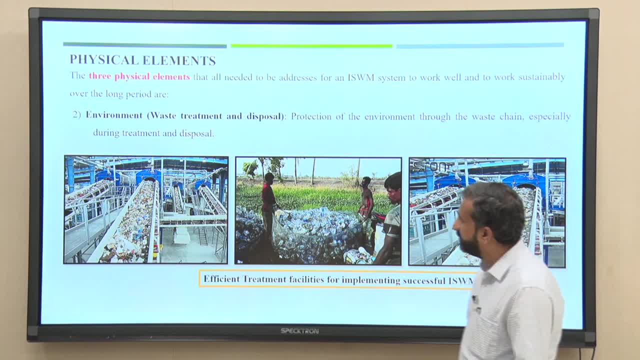 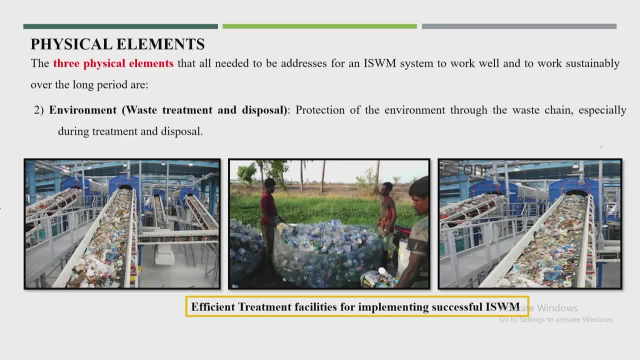 So by proper protection of environment through a waste chain, Especially during treatment and disposal. So if you have these kind of recycling process which I showed it in the some photograph, proper recycling process, proper treatment process, proper sanitary landfill facilities is available in the city so that we can easily maintain the environmental condition in the 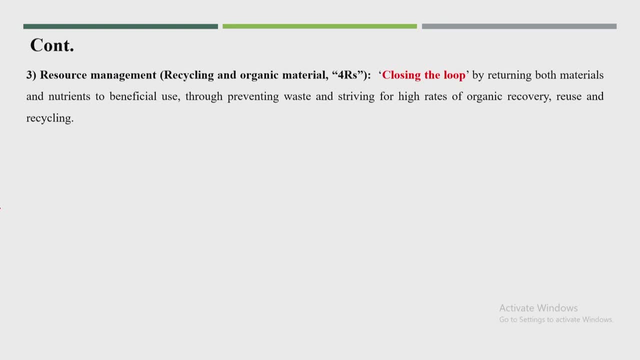 local area. And third point is the resource management. This is also one of the most important physical element of ISWM And this is also one of the most important physical element of ISWM. And third point is the resource management. This is also one of the most important physical element of ISWM. 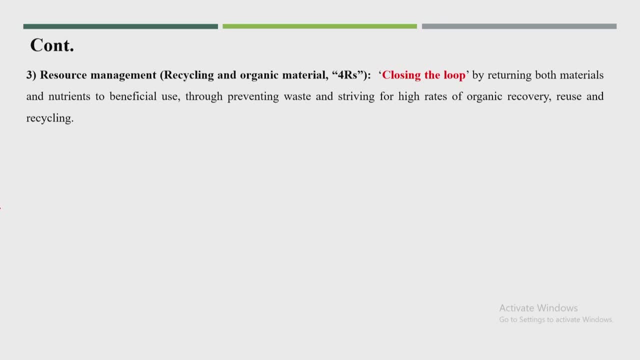 And how this resource management could be possible By proper recycling of dry waste and also getting product from the organic material. So in this one, if you talk about the 4Rs- normally we know the 3Rs, which I am showing in the next slide, the 4R- and closing the loop by returning both material nutrient to 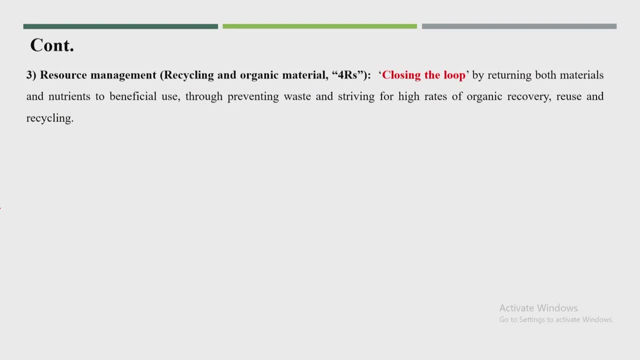 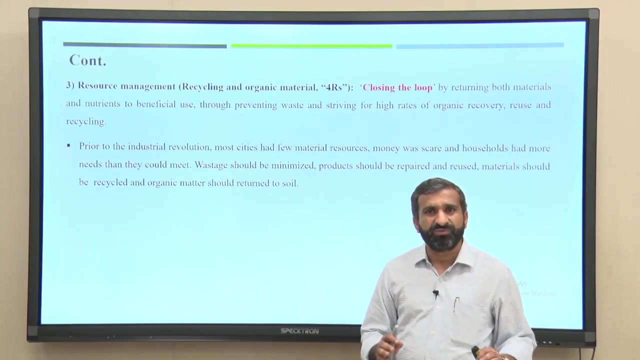 the beneficial use through preventing waste and striving for high rate of organic recovery and reuse end. So these physical element normally see, when you talk about the solid waste management plan, normally we will talk about the collection, we will talk about treatment, we will talk. 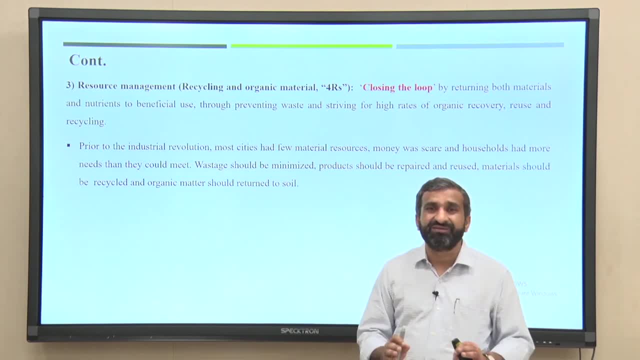 about disposal also, but these kind of physical elements is not possible until you will talk about the resource management. okay, because there are a lot of materials are getting recyclable, a lot of material can be treated and to get product out of that. so that is the important. 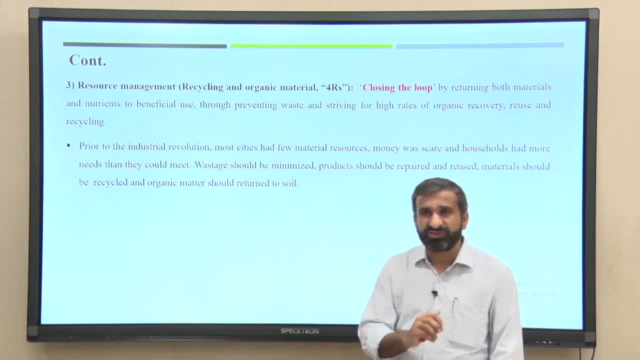 one. Now, when you talk about the treatment, also always thought about what kind of- or how best you can get it some kind of resource out of that, Like, for example, all most of the dry matter like metal, glass, paper, rubber, leather. 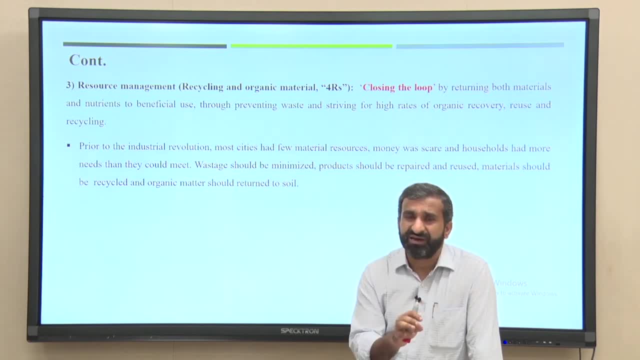 this is all recyclable- Okay, All recyclable one, and this is also become a one of the very good resource out of that- and most of these materials are combustible also. you can get energy out of that. that is also another one kind of very good product will come up out there, or resource will generate. 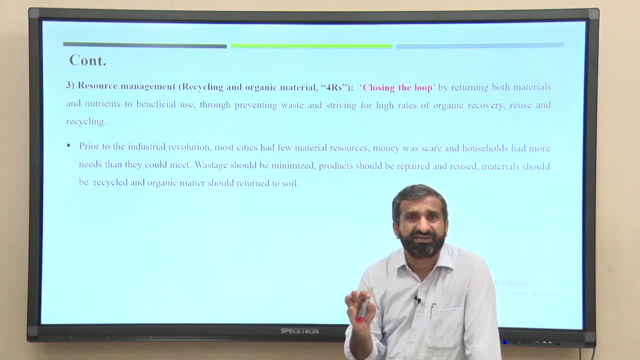 out of that and when you talk about the biological treatment processes. So in the composting, obviously we will get very good quality compost. if you are able to manage proper composting plant. In anaerobic digestion you will be able to produce methane gas. this is also one very 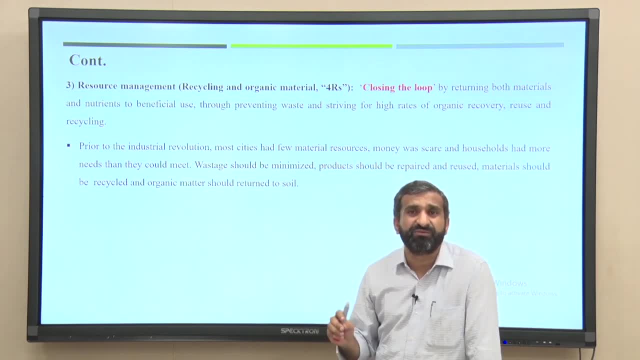 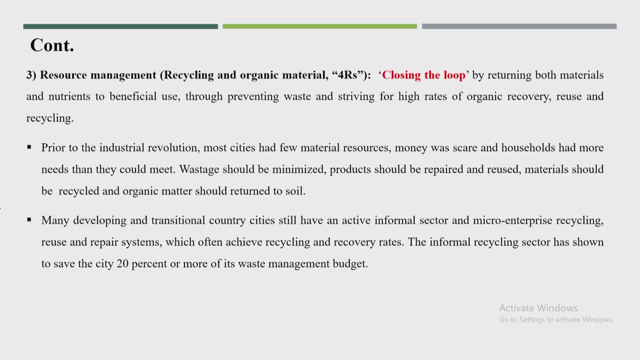 good way, very renewable kind of energy will be able to produce out of anaerobic digestion process. So almost all kinds of treatment processes or recycling processes will be able to produce resource out of out of that. So normally these resource management in most of the city is is not done by the formal 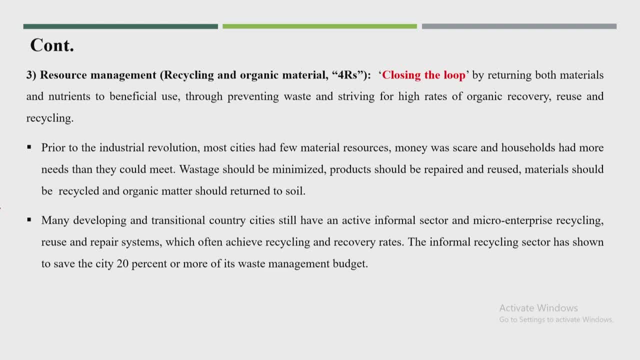 sectors. It is done by the corporation because they will be all busy with the collections and disposal only but they never and that kind of funds also has not available with them. But it is good. and the Swachh Bharat Mission- most of the cities got good amount of fund. 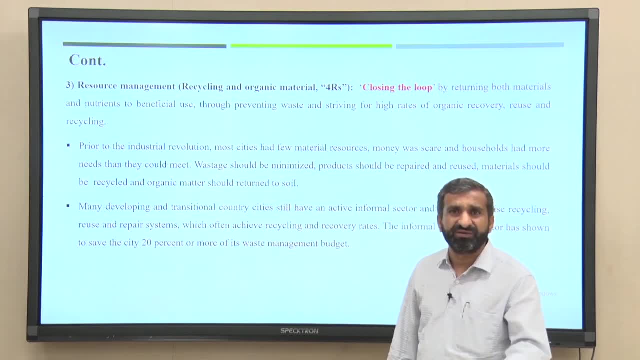 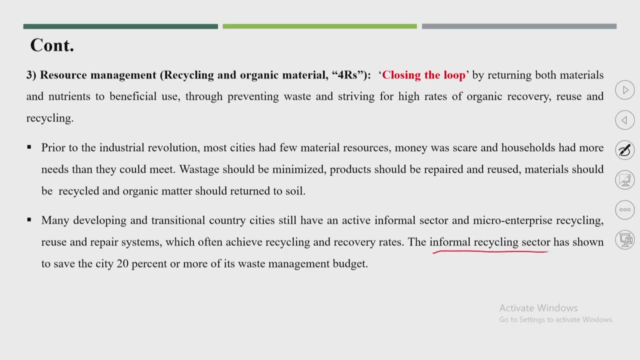 So let us see that many cities will come up with treatment facility or proper disposal facility. but on right now, this informal recycling sectors are sectors is around saved 20% of more waste management budget because there are a number of recycling facilities are available from the informal sectors. okay, 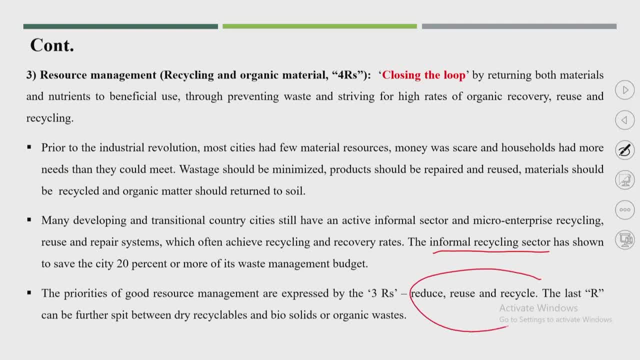 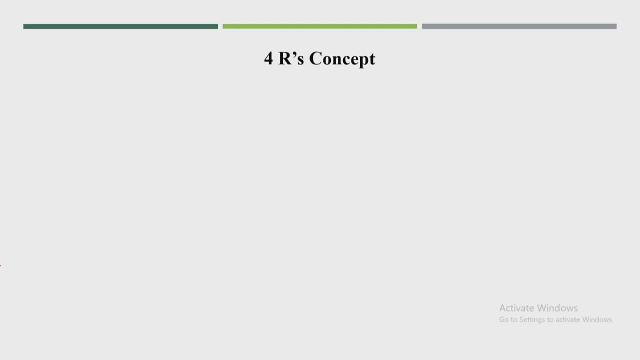 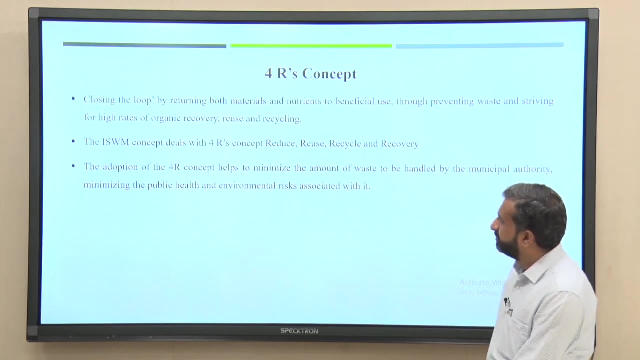 So the you know the three R's is a: reduce, reuse, recycle. okay, So this is the four R concept. normally this fourth R is specially given for the developing countries, specially like India, So close to that, Okay. Okay. So closing the loop by returning both material nutrient to the beneficial use. 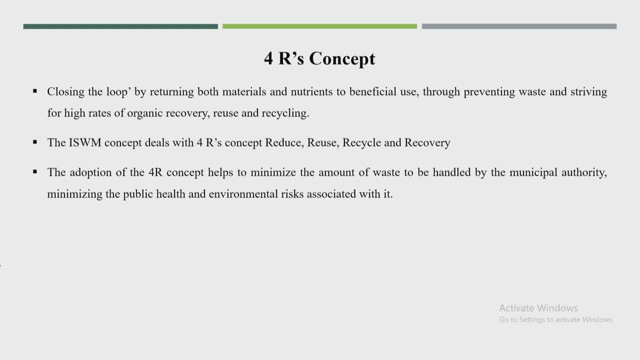 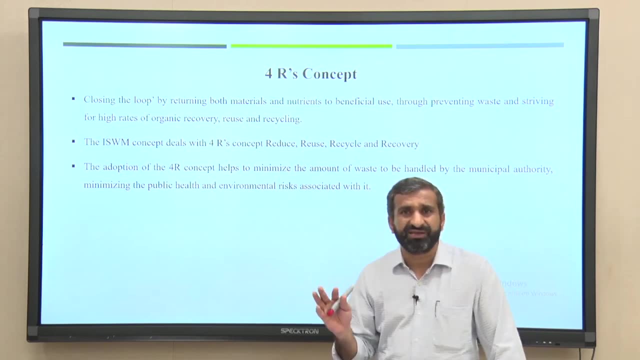 So this four R, the four R's means the first is the reduce as possible as reduce, reuse as possible as possible and recycle. and now the fourth R is a, is a special. this, this loop, will get closed by returning material or nutrient to the beneficial use. 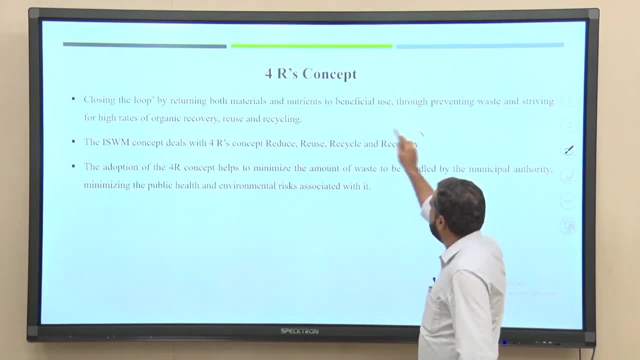 These are especially. I think many, I think many, many textbook you will find is a recovery. they are writing so, but I think I would not. I put it here because most of the textbooks also you will find this recovery one. but see, this is recycle also is one kind of recovery. these, these, rather than recovery. 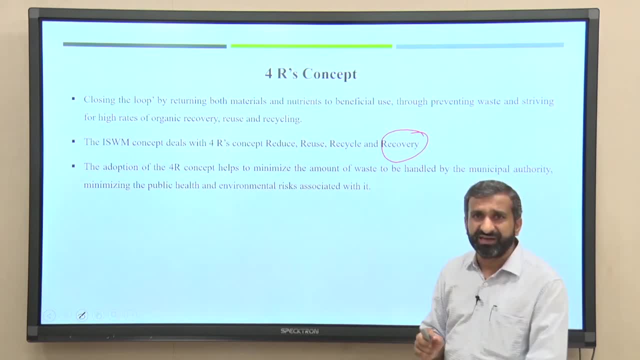 the important thought about developing countries like India. this R is for return nutrients to soil. Okay, This is the best word. in the by. by R, there is return nutrients to soil. means what is the? what is the definition of that? how the nutrients will be returned to the soil by. 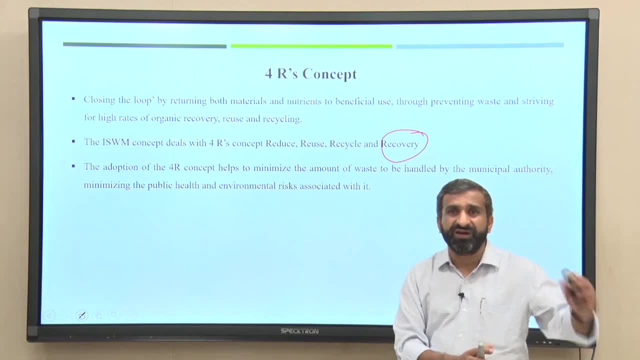 producing compost. compost from the wet waste of the. these compost will have a lot of nutrients and these nutrients is getting returned to the soil because the the same waste has been generated in the soil And a lot of nutrients took from the soil and to come up with the as an food for the. 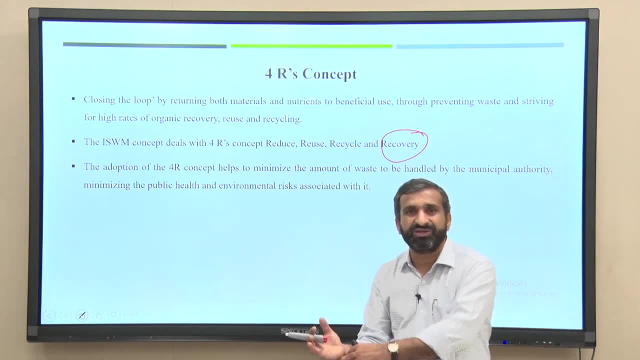 humans, So why not? the same nutrients we need to return to the soil, So that is a good idea for the developing countries like India, even the, the South Asian countries or even the African countries, if if this kind of idea is is very, very important. 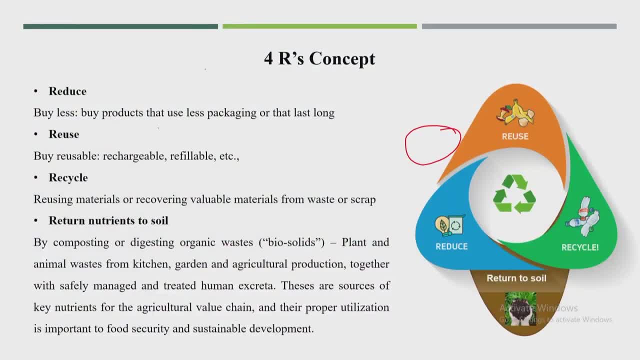 to propose. Okay, So it is a reduce, reuse, recycle and new, return nutrients to soil. So by composting we can easily, we can have the these particular nutrients. we can also return to the soil. So it will close the entire loop. 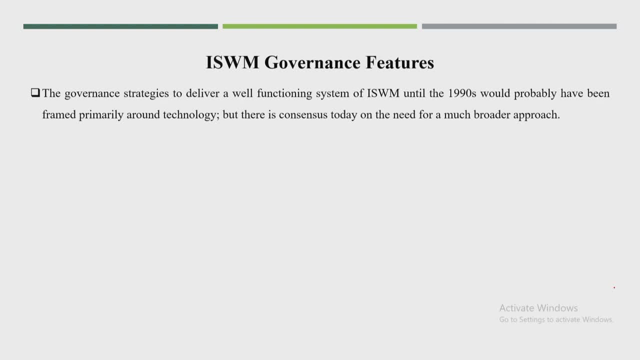 Now the governance features. So there are three governance features. Okay, So the governance strategy to deliver the well functional system of ISWM until the 1990 would probably have been frame primarily around technology. but there is a, there is a need. 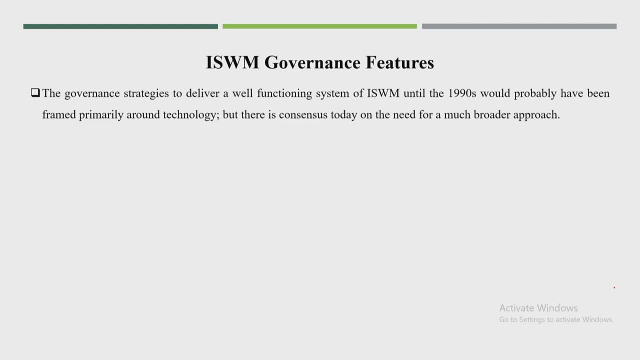 of governance, government participations also is very important, or some of the governance features also are important. So this is the one that earlier, even 90s, 90s It is. we always talk about the technology. we required special technology for treatment of mixed base. 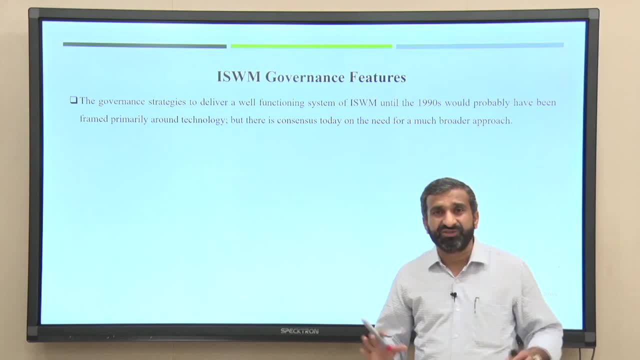 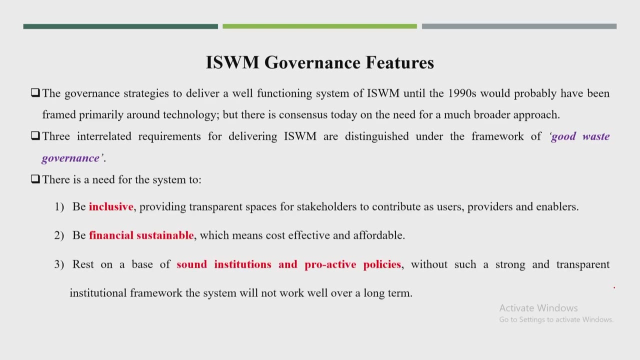 Likewise we used to discuss, we never used to talk about, some governance features also are important to to have the proper management system. So this good, best governance. there are three major governance features. First is the inclusive. So is a inclusive providing the transparent space for the stack holder to control the 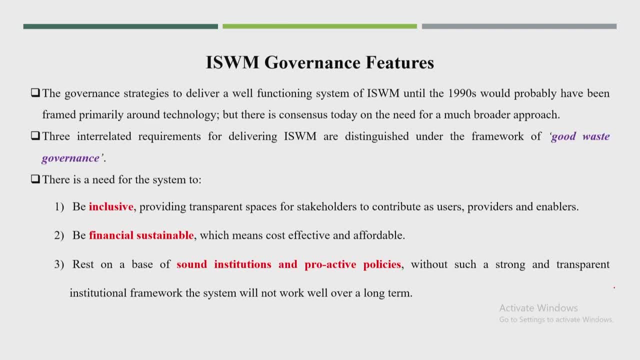 stack holder contribute as user. Next is the financial, sustainable. and third is the sound institutions and proactive policies. Now here you understand that it should be. whatever plan you make it, it should be inclusive. So what is the meaning of inclusive means it should be contribute. 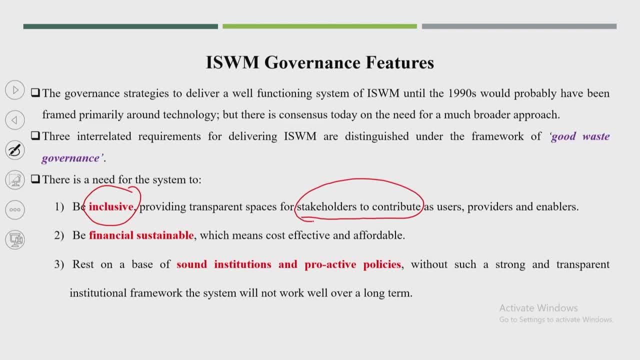 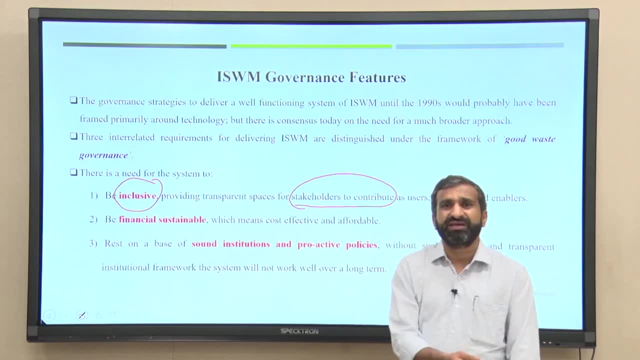 by the all the stakeholders. This is the one of the very important point. Now, what is normally the plan is proposed by the local authority that how best they can collect the waste and they can dispose the waste, But I think they never talk about the generators. 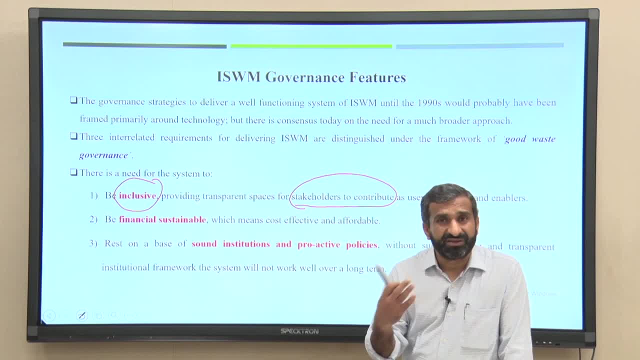 they never talked about the, the rag pickers or informal sector. there are a number of NGOs are working with the waste management. they never used to talk about them So many times. see, suppose some corporation is starting some initiation facility. they never thought. 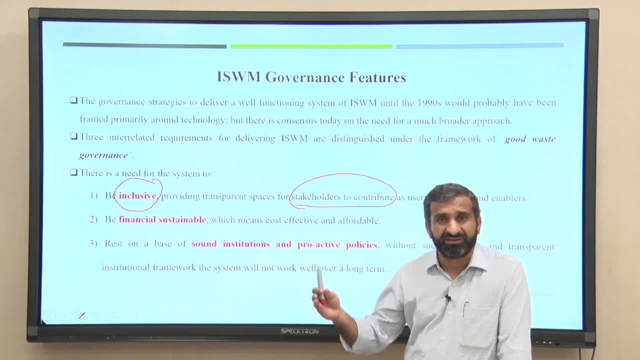 about the waste management. So there are hundreds of rag picker. they are continuously collecting, or from last few years they were collecting the recyclable matters for, and so suppose, if you have the one particular incision plant so they they would not be able to collect that waste. So 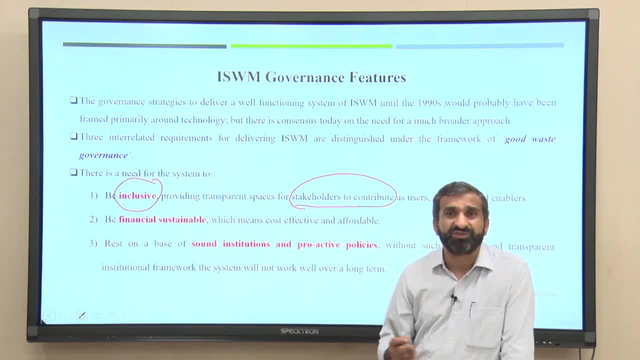 I think you need to have discussion with them also. their inclusion also is very important. Next is the financial sustainability. This is very important one. See any project. if it is not financial sustainable, how we can extend that project for 20 years or 25 years. 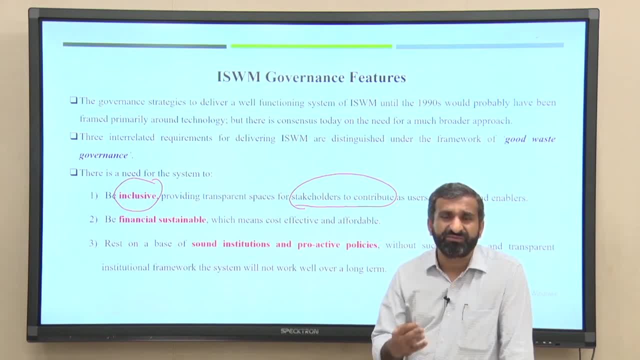 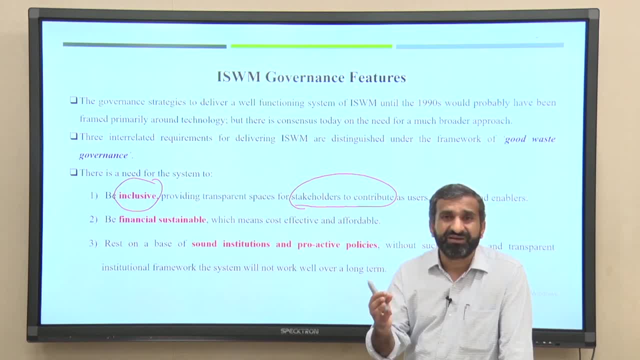 you know, But that this many of these are what is alright, if you get some out of some kind of fund out of that can generate fund out of that biogas. see, you can install the biogas plant and you are saying that our city is having very good biogas plant, very big. 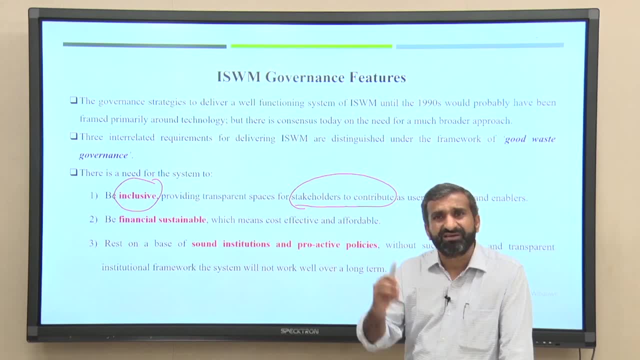 biogas reactor we have been installed biogas is producing, And if you are not able to utilize that particular biogas for energy production, what is the benefit of such kind of plant? But the you can say that you reduce the waste or you maintain the waste by having this kind of. 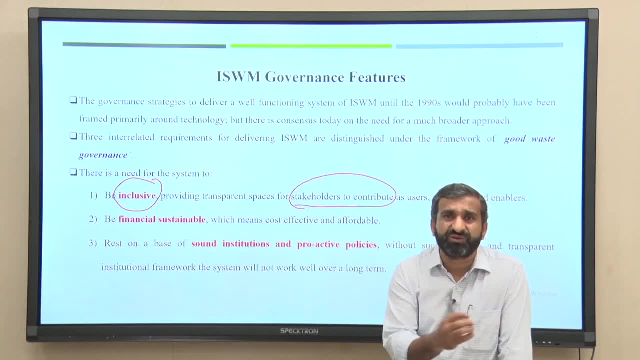 treatment facility, but how these plants will work for next 20 years or 25 year, Because the obviously capital fund you cannot generate by selling of this kind of product, but capital, capital fund. you will get it from the either state government or central government. 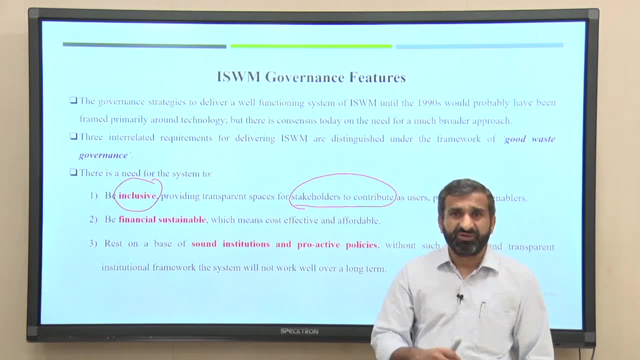 to have such kind of facility, but for operation cost, because for all this kind of treatment process you will be required a lot of man powers, a lot of maintenance issues are there. So you will be required fund now every year. do will you ask the? these corporations will. 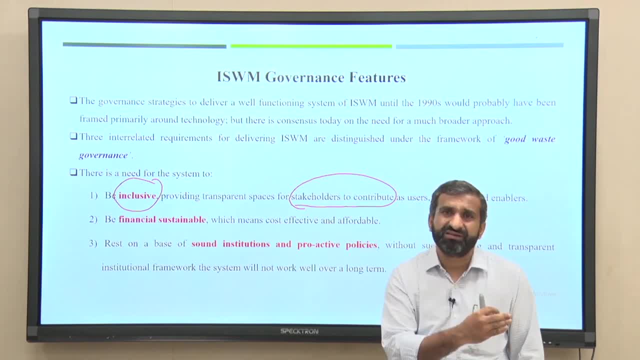 ask the fund to the state government or central government. no, they have to depend on their own, so that financial sustainability has to be there. until now I never saw that any corporation is talking about the sustainability. So maybe sustainability cannot possible in first five years. Maybe the sustainability will come by next 10 years, no issue, but at least you are trying. 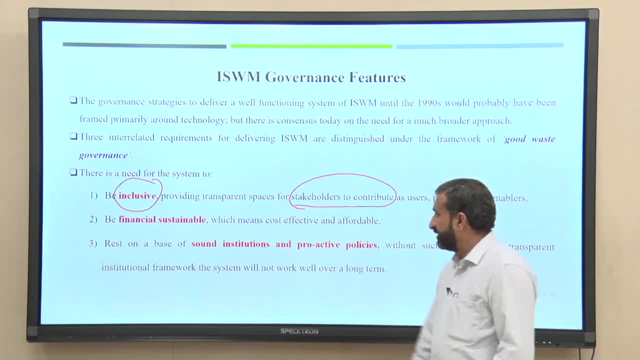 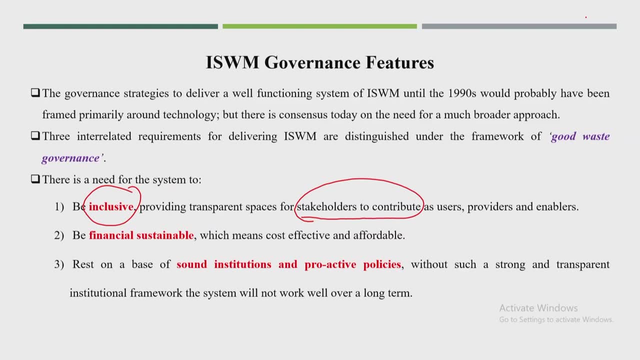 to be become sustainable. So that is the idea. next is the sound institutions and proactive policy. This is another very important the governance feature. So in India normally we do not have sound institutions. I think you can. you can say that we have Swachh Bharat Mission started. 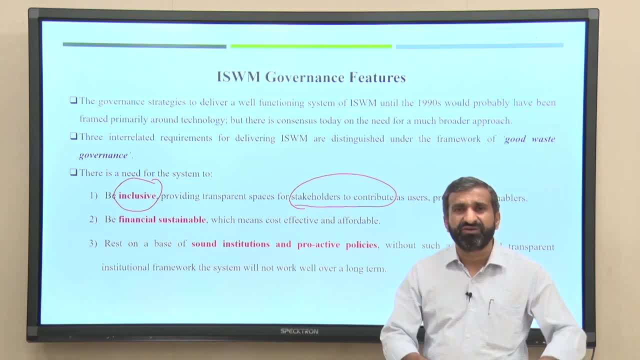 By ministry. but these ministries are working for working for total environment. The rules are making by the one special ministry called Ministry of Environment. They have there. but we need sound institutions, We need some special institutions or even the academic institutions also. we do not have 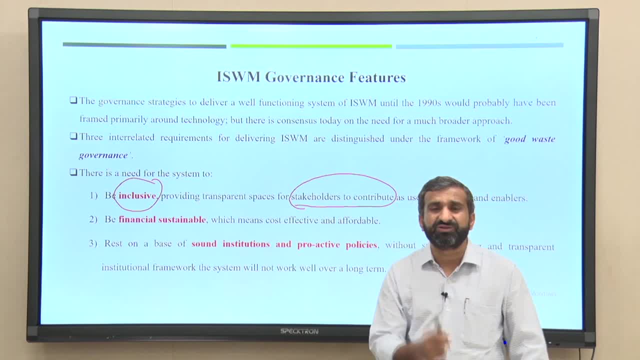 like. did you find anywhere the, the special degree on solid waste management, For even the for solid waste management also, I think these, these course, to study these course you have, you have to get admission in IITs or very big institutes in India, after passing the gate exam in the very good score. then only you will get admission in such colleges. 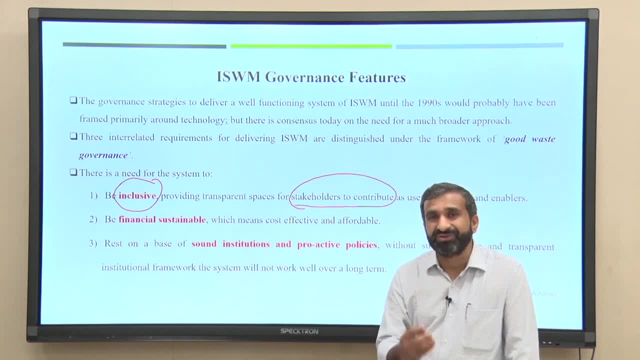 and then only you will study these kind of courses. So so you, you, you required. And problem is there Is that, see, a lot of man powers are involving into the solid waste management programs. but we are those, those man powers are skilled. No, they, they are, they are they, they, they are learning by working in the plants. 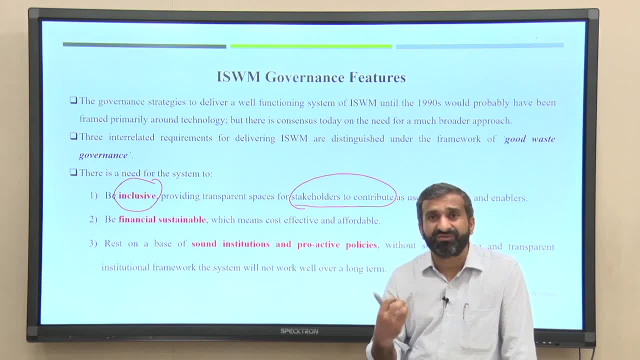 So they, they do not have skill. So for skilled you required special institutions to to create the skill in the those man powers, And also you we required special proactive policies. So every year need to get some fund to the local authority, is not that once in a 15 years? 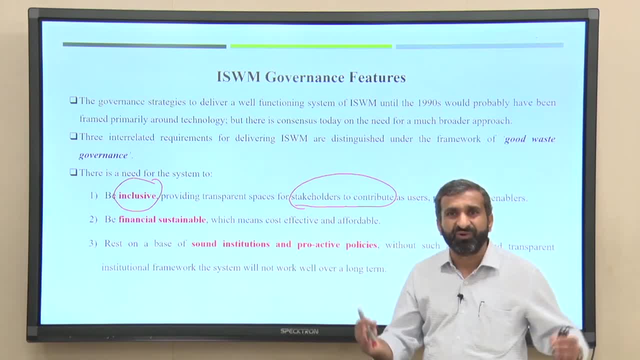 once in a 20 years you give one capital fund, maybe a few crores, and ask the local authority to start some plants and run it for next 20 years is not possible because you need continuous fundings. also should be available. So So until that. 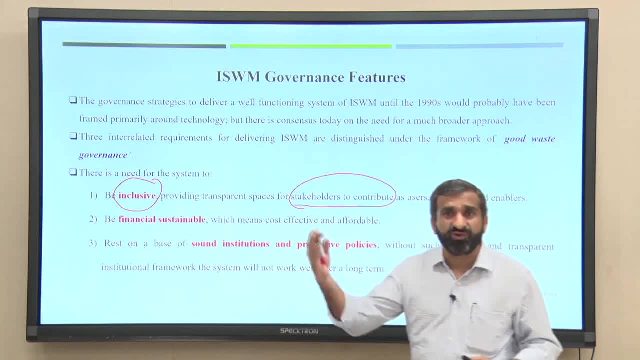 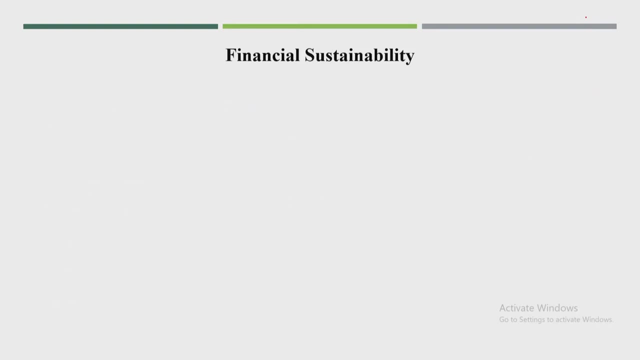 Until the, Until the local authority won't go for sustainability or won't achieve the sustainability, until that you need to fund them and particular policy should, should be required. So same thing here also. I wrote it, You can read this: So financial sustainability. 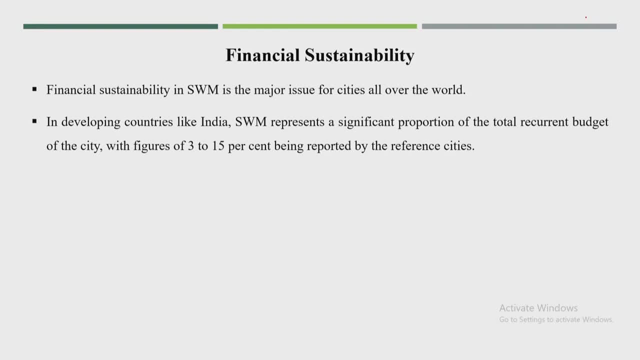 So you can see here, in developing countries like India, SWM represent a significant proportion of the total concurrent budget of the city, with figures Of 3 to 15% being reported by the reference city. And if you see that when the solid waste budgets are divided by the population, this per capita. 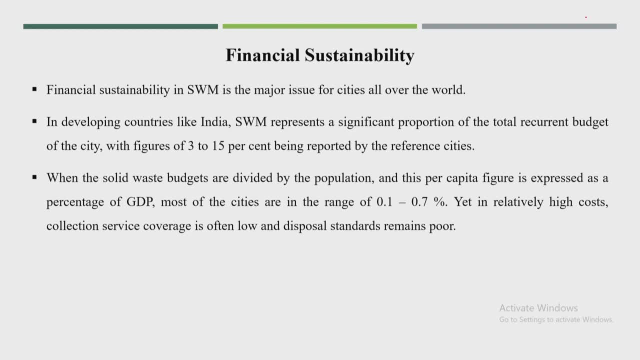 figure is expressed as a percentage of GDP. Most of the cities are in the range of 0.1 to 0.7%. 18- relatively high cost collection services coverage is often low and disposal standard remains poor. See This is the one problem with the financial sustainability. 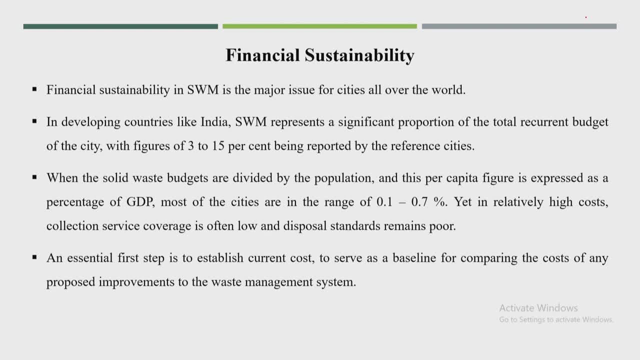 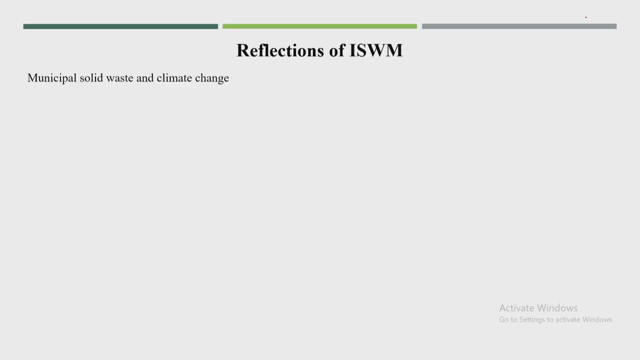 So the essential first step is to establish current cost to serve as a baseline for comparing the cost of any proposal improving improvements into the waste management system And similarly sound institutions. Now there are some reflections of ISWM with the solid waste, municipal solid waste management. 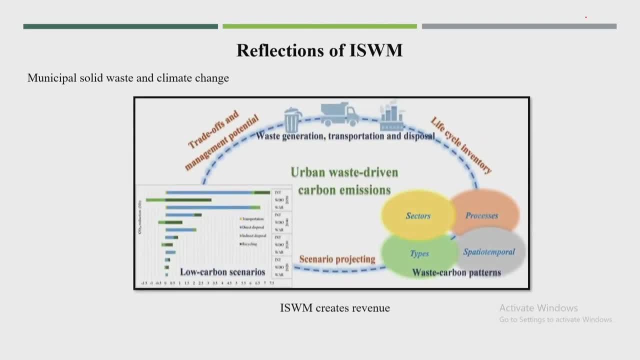 And with the climate change also. So obviously I think if you have proper solid waste management plan and or integrated solid waste management plan is obviously you can reduce the carbon emission and because of we can get a lot of fund by low carbon scenario because of that and waste recycling. 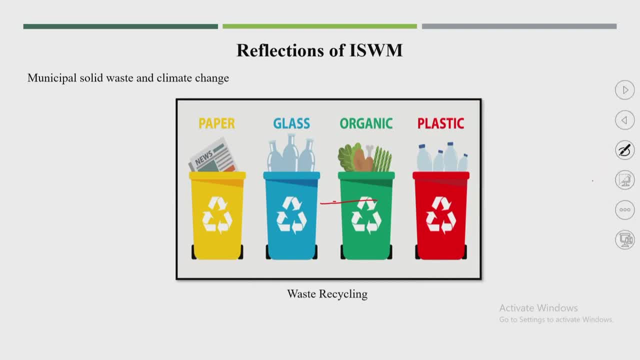 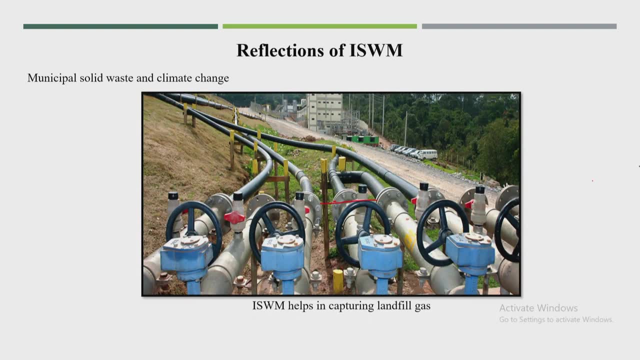 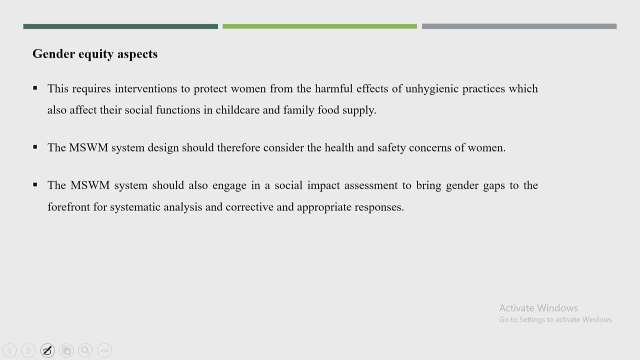 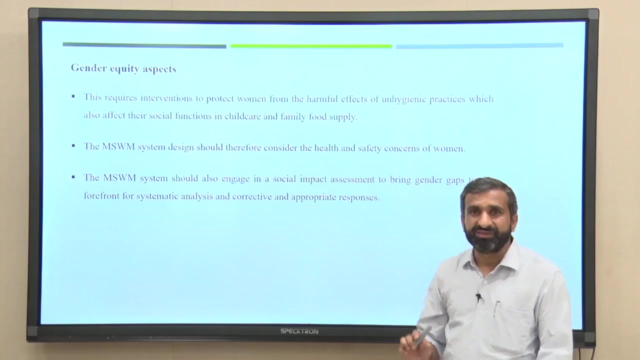 So obviously we can reduce the, We can maintain proper climatic change by waste recycling, by capturing landfill gas, So that the it will not create problem to the environment. Now this is one slide- is for gender equity aspects. I think this slide- I keep it here based because in solid informal sector, especially if you 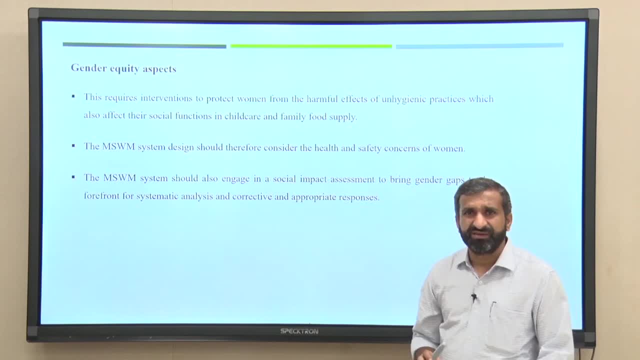 see that number of females are working In the In the solid waste management and even the kids are working for the solid waste management system. So under the integrated solid waste management need to be designed in such a way that the proper gender equity aspects we can maintain. 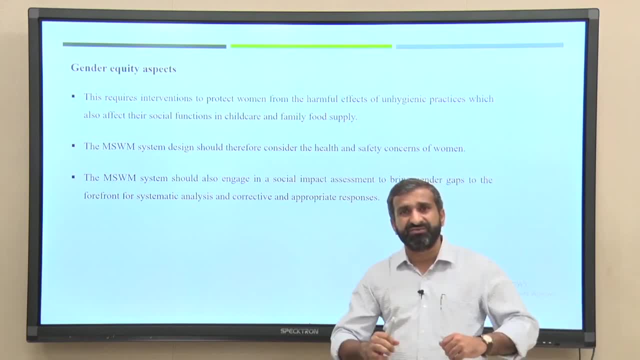 So is not only the only the males are working for the waste management and females are not working. Only females will work for street sweeping And they should not be allowed. They are not allowing at disposal sites. It should not be like that. Try to maintain the the female equity, because there are number of man powers are working. 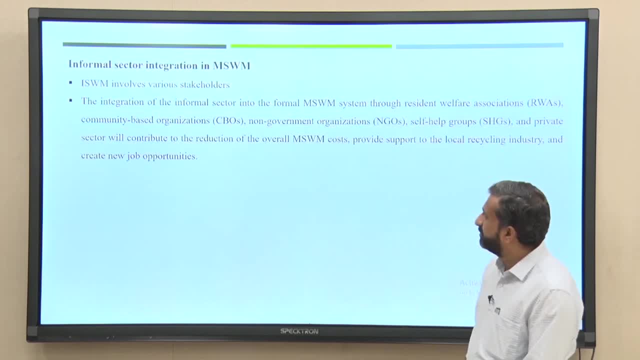 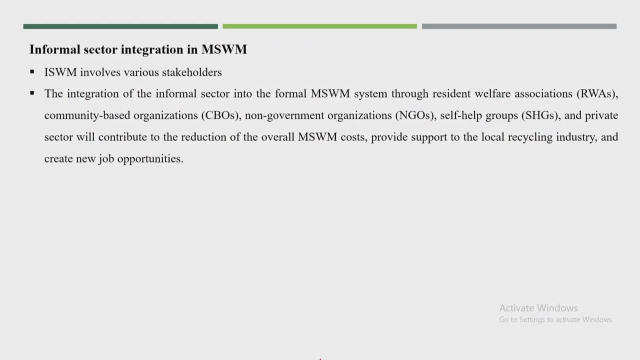 in the solid waste management projects. Similarly, the informal sector integration. this actually we have seen in the governance features also inclusive. So in the inclusive is not only the, The governance features, The government participation only or government companies or governments, authorities participation only should be inclusive. 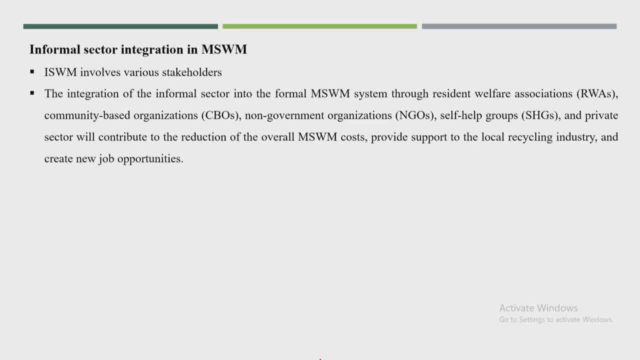 But also the informal sector also should be integrate, like NGO, CBOs, community based organization, self help group, some private sector. Now here in 2006, when this PPP projects have been started under JNRM program, So there also This discussion had been started. 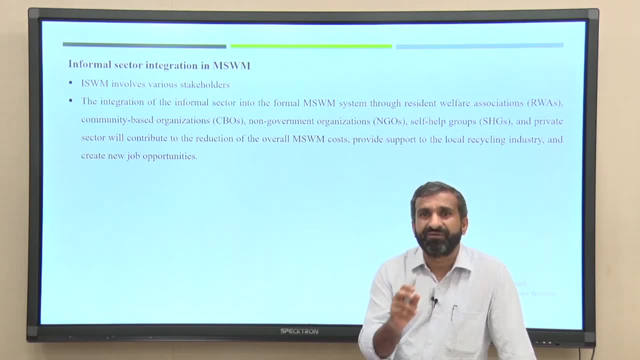 So there, when you say PPP projects means public, private partnership partnership. So public means is a local authority, local governments, and private means is a private company. Now, when this discussion had been extended, there also this question has been come up. only the these collaboration is between the local corporation and with the private company. 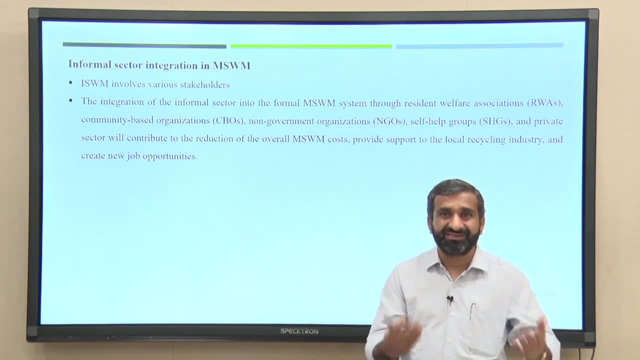 What is? what is the role of other stakeholders Like Like generators, The household people or enablers, they also need to be include into that. So that is why the the- this was one second- the rag picker. We have huge population in the city of the rag picking. 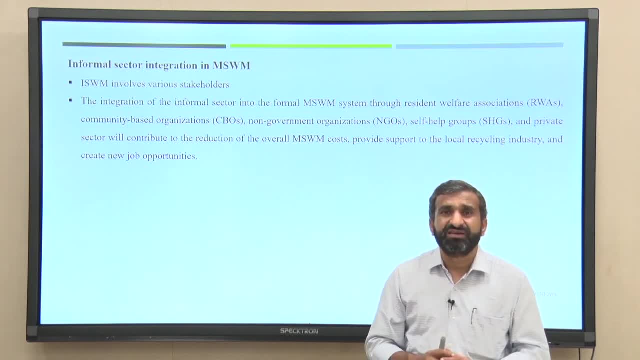 There are number of NGOs are working, CBOs are working and self help groups are there, So they also need to be, at least to come up into these kind of programs. So I personally believe that, like in NGOs, these, these are also the big groups. 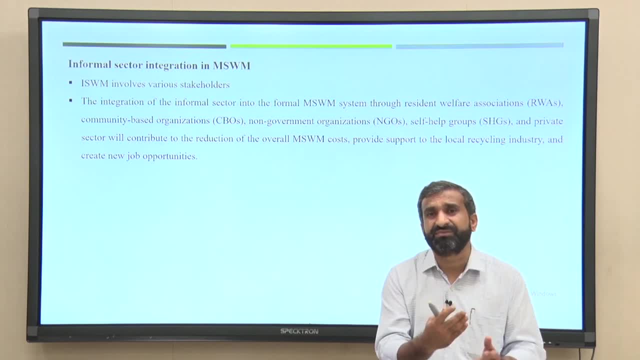 Why not? these NGOs can be, can be accept as an in the primary collection. Maybe they cannot go, cannot go for treatment and disposal facility because it is a very big, big task for them, But at least for for primary primary collection they can help under why why I am proposing: 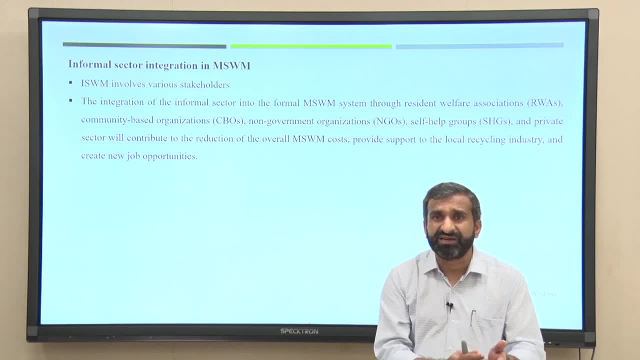 that NGOs in the primary collection, Because for primary collection you need to aware the local people first, and aware is not only to provide the proper waste but also to provide the segregated waste. So you will be required lot of awareness thing, awareness issues required. So why not? by giving that particular task to the NGOs, they can also go for awareness. 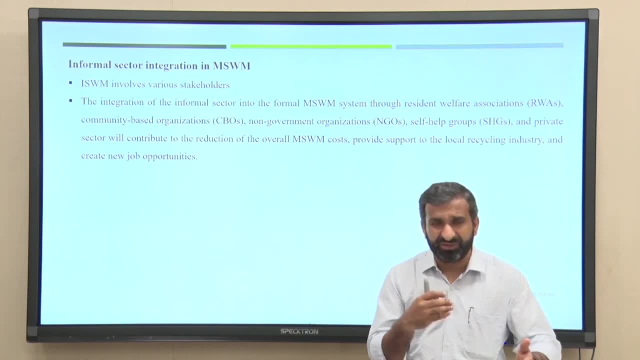 awareness first and they can talk to the each household, households and can explain their problem. What will the benefit of segregation? how base they can do the segregation in the house. So that kind of integration should be, should be required, And also because now these informal sectors are not coming under the official jobs. they 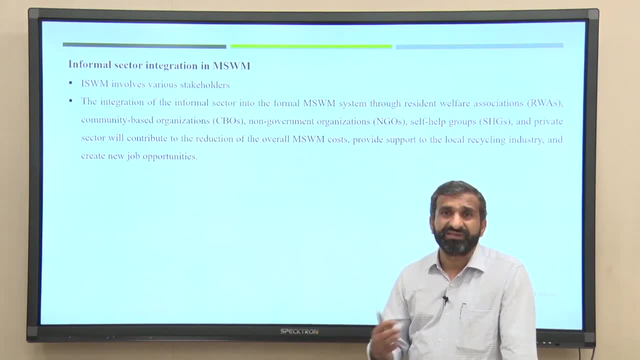 because they are in the informal one. So why? by giving this particular task to them? like that, there are a number of rag pickers If you have one particular kind of recycling facility near the disposal site or maybe somewhere somewhere very close where number of rag pickers are residing. 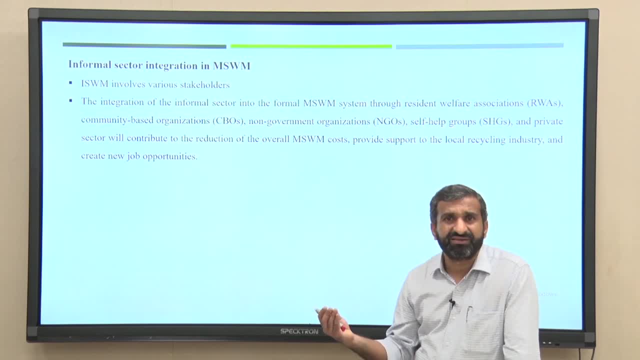 So and ask them to get collect the recyclable matter, and by that way we can pay them, we can give the proper jobs to them And because of that you can ask them to proper, have proper clothes. You can provide them shoes, Shoes And all the facility you can provide them. 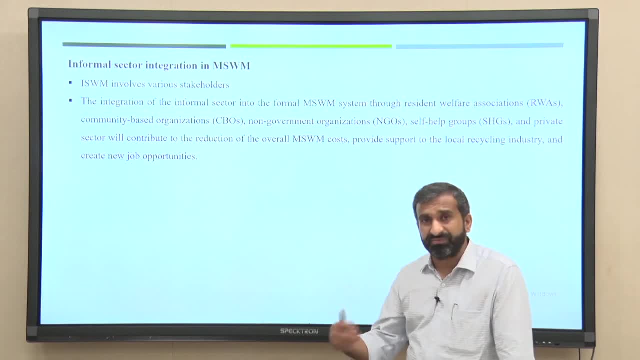 So they will also enjoy and they will also work for you and but pay, pay properly to those people. So in they, they, they will be also also also can accepted as an, as an one of the work, working person for the, along with the local authorities. 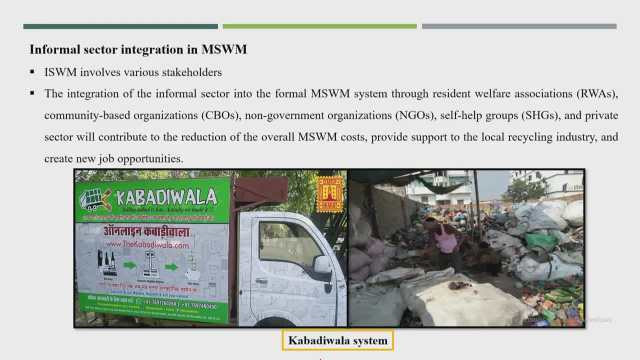 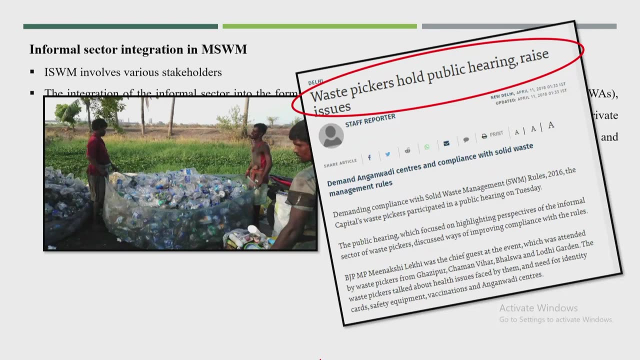 So likewise here. The Kabaddiwala system- So there are, number of Kabaddiwala are there, So why not? you can include such kind of people And also the. this is one news. that way, speakers hold public hearing, raise issues okay. 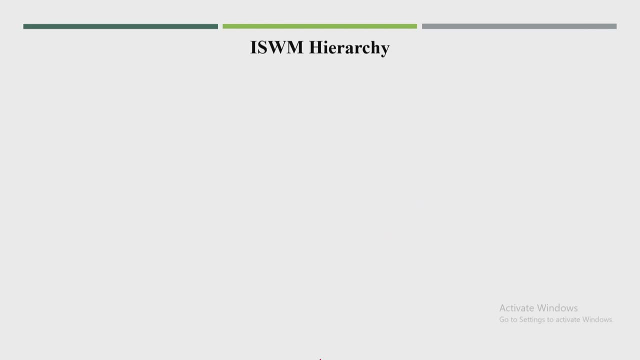 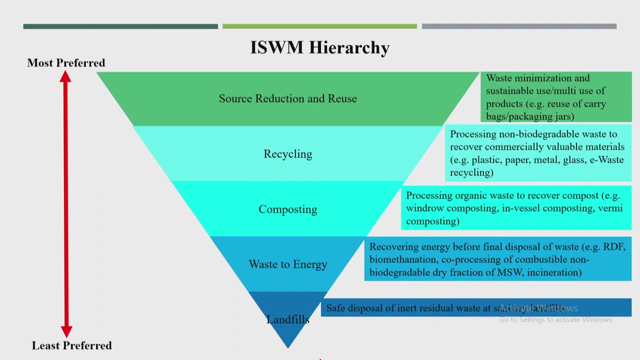 Now, when you talk about the hierarchy of integrated solidarity, Okay, Okay, Of integrated solid waste management, what should be the hierarchy of integrated solid waste management. So this is the most preferred to the least preferred hierarchy of integrated solid waste management plan. So now here. first, start from the source: reduction and reuse. okay, 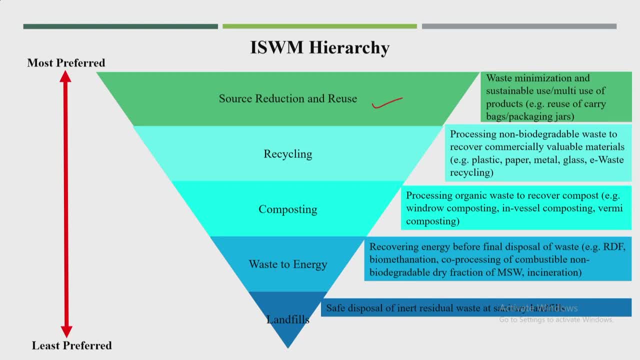 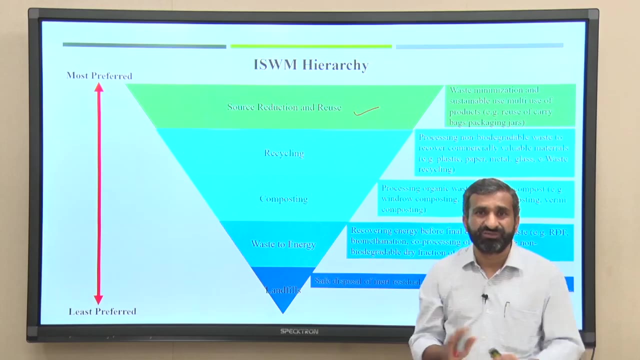 This is the most preferred the point, followed by recycling. suppose now when you make a plan. So first you talk about how best you can reduce the waste, reduce or reuse the waste. that is the first thought should come to your mind, or come come to the local authorities when 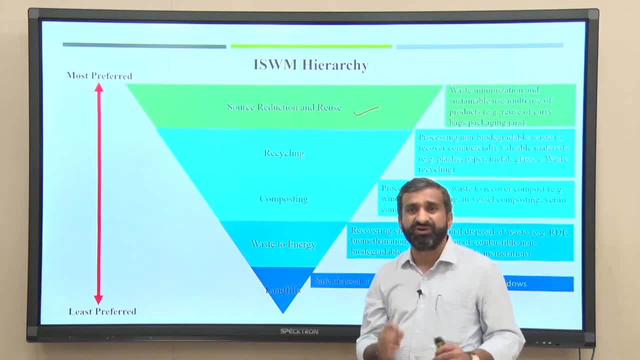 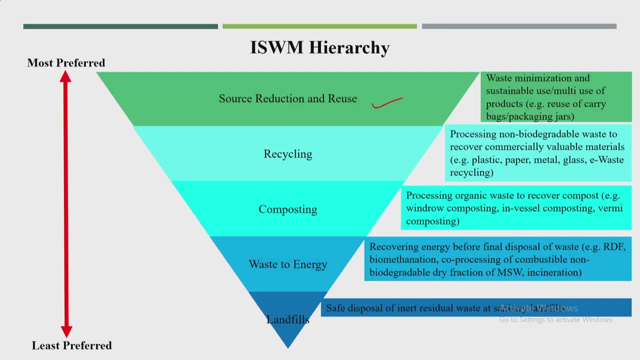 you are, they are planning for solid waste management plan or integrated solid waste management plan, Then how best they can go for recycling- recycling of all valuable matters, and then, once the once, whatever best could be possible to reduce, reuse And recycle. then you talk about composting the all your biological waste. how best you. 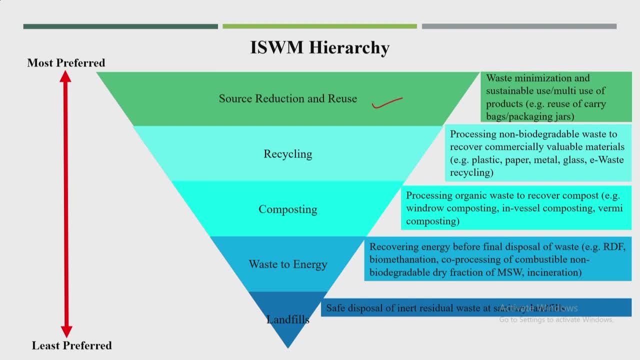 can take it out and go for composting process. may be composting or biogas facility, anaerobic digestion facility also. you can thought about, think about that and then then finally go for either waste to waste, to energy, if possible waste to energy and now waste to energy by 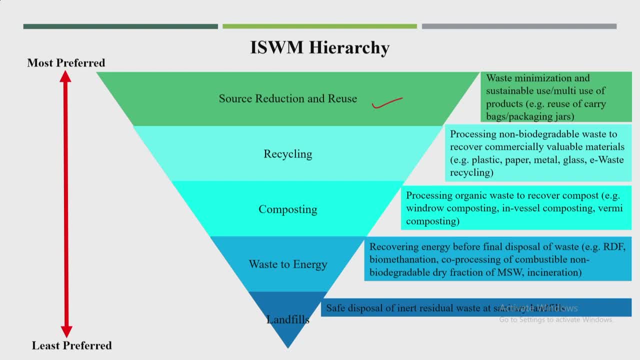 that we can get some kind of energy, may be the, even the, under this biomethiation or anaerobic digestion. also, you can propose under the waste to energy. if finally go for landfilling which is the least preferred, okay. So whatever is not possible for source reduction, not for recycling, composting, waste to energy. 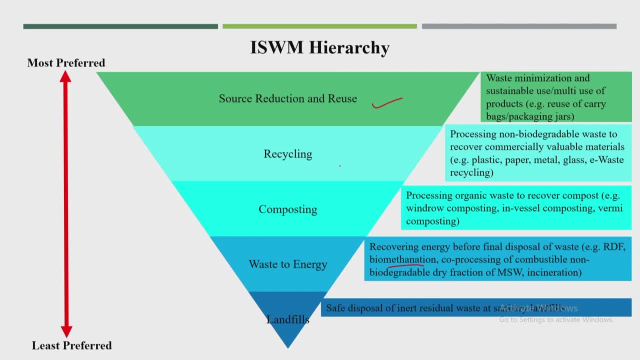 that will go to the landfill area. That is the least preferred. Okay, So that is the proper hierarchy of the integrated solid waste management strategy or plan. But in India I think, rather than discussing on this, will directly go for landfill, So will first most preferred is the landfill and then. then we will talk about the recycling. 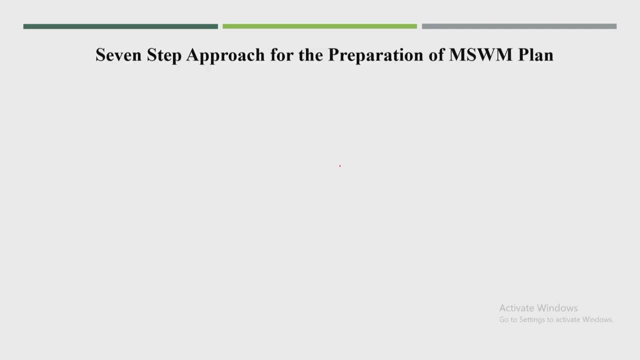 composting or waste to energy. that is not the good idea. Now the seven step approach for the preparation of MSWM plan. Okay, So this particular plan has been proposed under the solid waste management plan and I found is very good. So I will just share few important points. 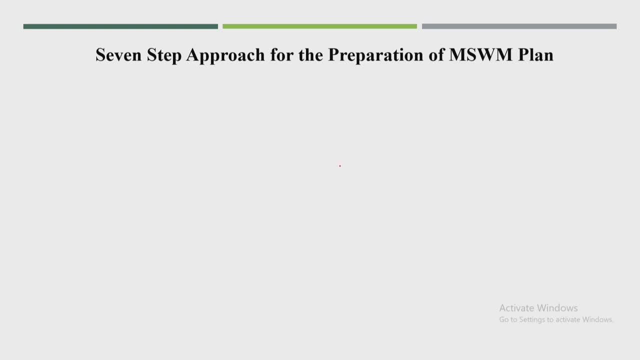 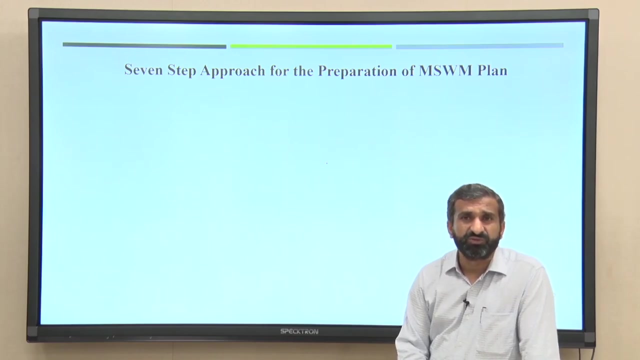 So this, actually this approach is. I personally believe that is very good for the corporations, because in India there are number of class two and class three towns where population is around 1 million, 1 million to 0.1 million. population is reciting like districts or taluka level and and if you 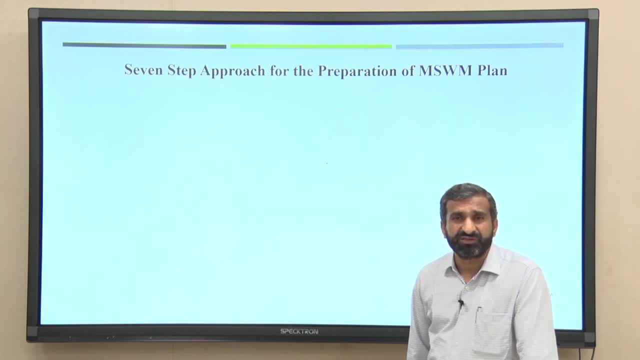 talk to them about the preparation of solid waste management plan. many of their staffs are not well aware about this kind of thing, the plan preparation. So this approach will help to those kind of corporations, Okay, Okay, So corporations where the proper- or maybe proper- staffs are not available to understand. 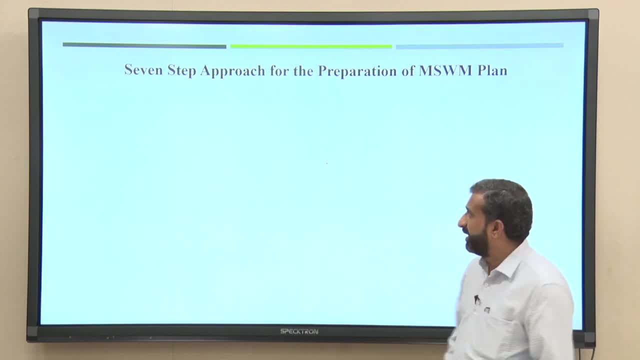 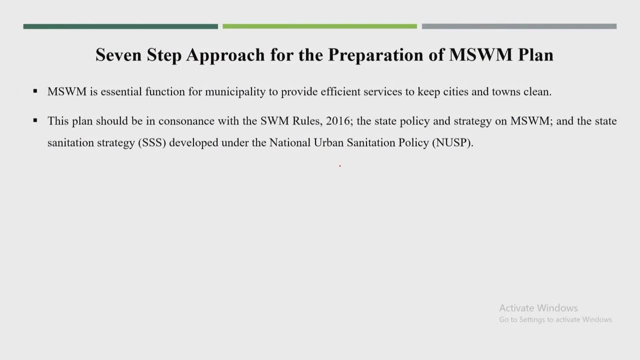 and by that way, they can come up with a particular plan. So these plans should be should be along with the SWM rule 2016 and and the state standard standardization strategy developed under the 19th century. So these plans should be developed under the national urban sanitation policy. 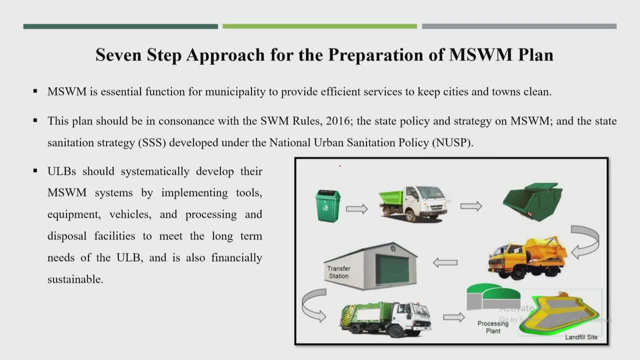 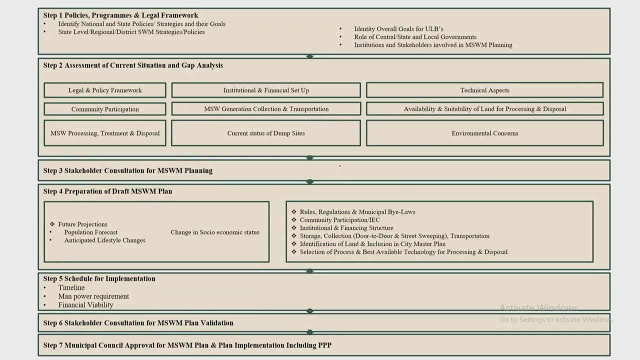 So ULB should systematically develop their MSWM WM system by implementing tools, equipment, vehicle processing and disposal facility to meet the long term need of the ULB and is also financially sustainable. So this is what the different steps. Okay, So step one is a policy program. 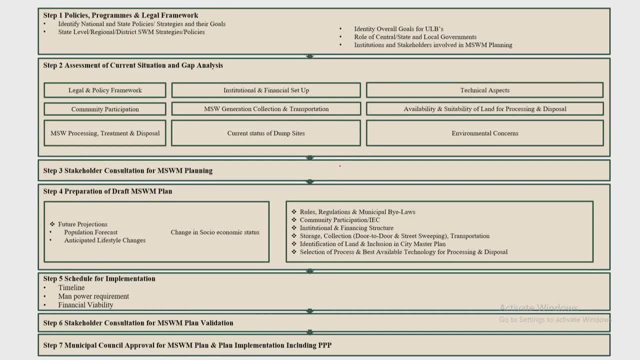 Okay, So step one is a policy program. Okay, So step two is a legal framework. Step two is assessment of current situation and gap analysis, And also the the stack holders is is given here in step one: what. what will be the stack holder in step two- assessment of current situation, gap analysis: what are the stack holders or? 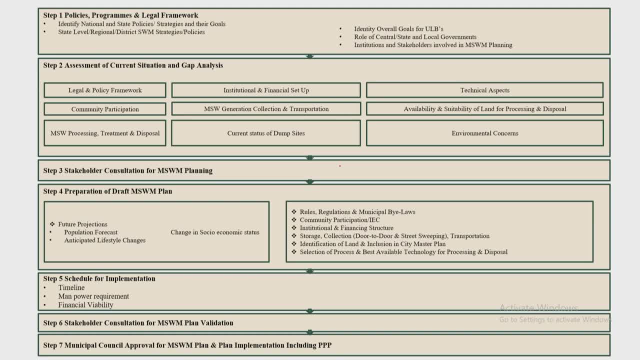 what are the aspects has to be look upon into this particular step. third is the step three is a stack holder consultation of MSWM planning. So here the third point: once you are coming with the assessment, current situation gap analysis will come up with the stack holder consultation and, based on the consultation, 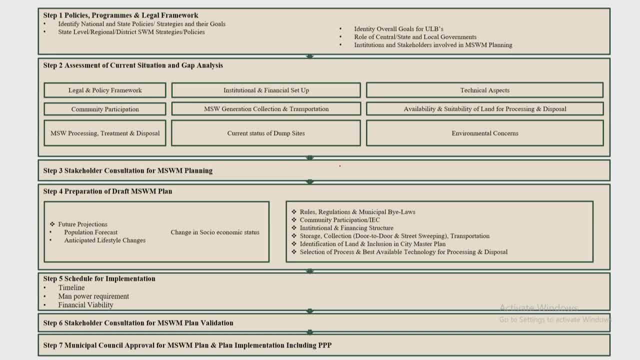 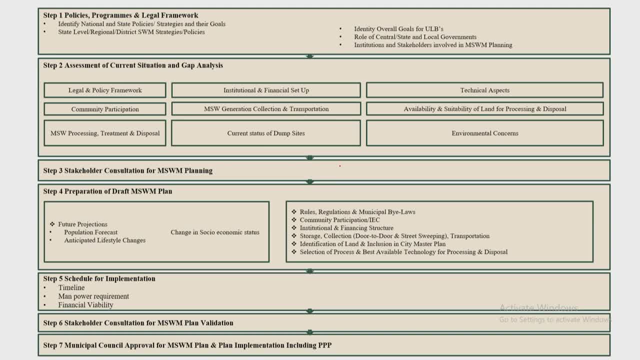 So timeline, manpower, financial viability, that will be become prepared and once the draft proposal with the schedule, again we will go for stack holder consultation. So again we will go to the step three and we will have discussion there with the all the stack holders and once everything is accepted to the all the stack holders will go to the. 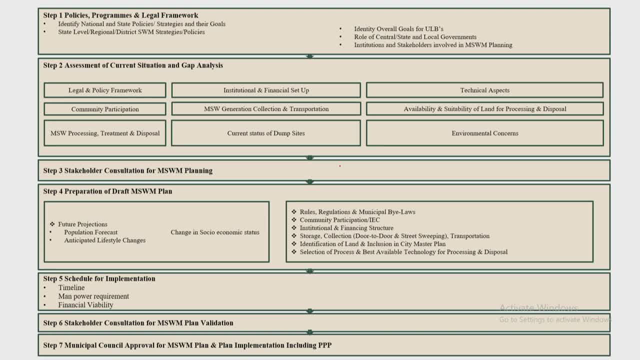 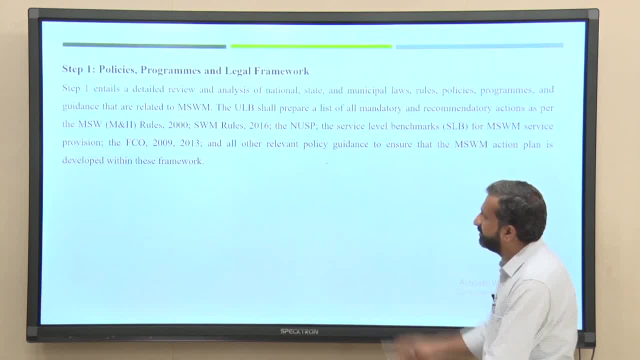 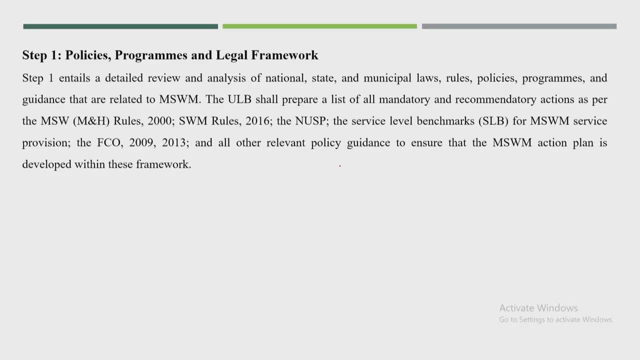 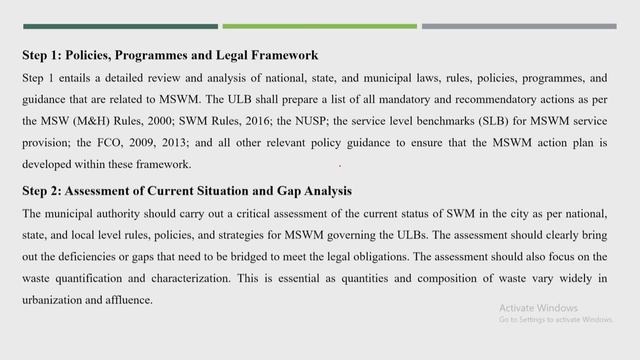 step seven: municipal council approval for MSWM plan and implementation, including PPP. So this also I explained in the step by step. So step one is for to create the policies or legal framework to the local authority. Step two: this is the important step. I believe that because before making any plan go for 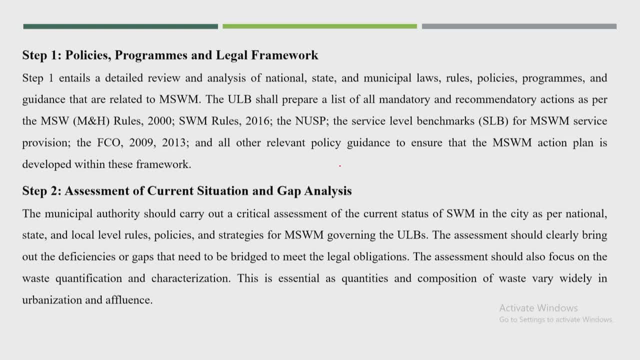 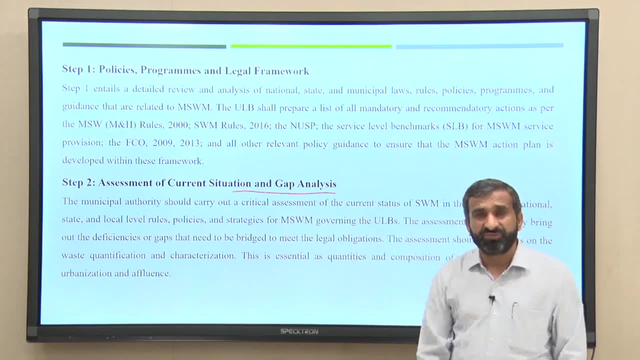 first, the current situation and gap analysis. Now here to assess the current situation. gap analysis: I particularly believe that the each corporation need to talk with some experts. These experts from the could be from the private, private enter, as in industries, or from the academic institutes also could possible. 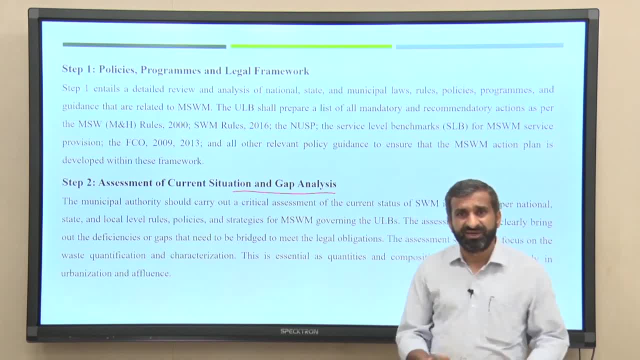 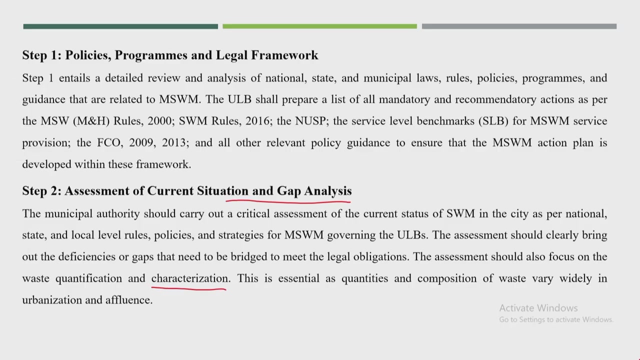 There are a number of Academic professors, like in the IIT or NIT or other central colleges or state colleges, where the researchers are working. I think, I believe, that, because there are a lot of data has to be collect and also the quantification and characterization study has to be perform, 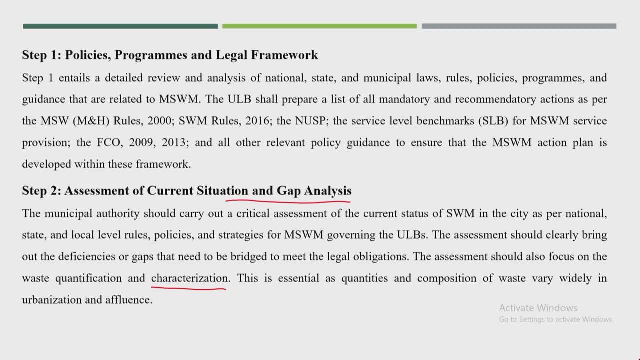 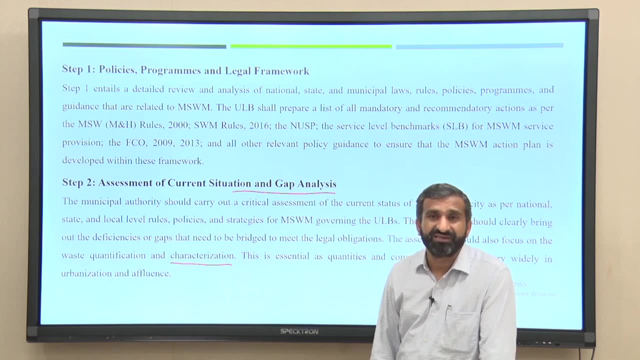 into this particular step, otherwise is very difficult to understand the what should be the current So situation and gap analysis is not possible. and this characterization also is very difficult. We have, we had a one module on to the characterization, So obviously I think if the local authorities involved some academic faculty or professors. 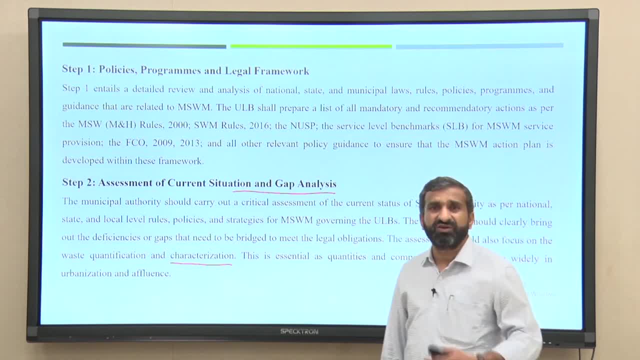 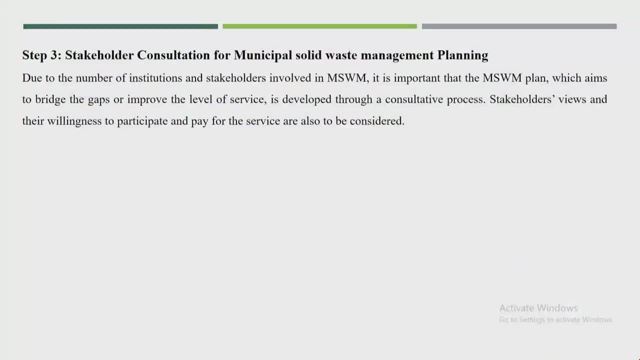 is good for their good. for them also, lot of discussions and lot of new understanding will come up in this step. So one, the step two is known. Then we can go to the Stakeholder consultation and talk to them. This is what the current situations are available under, as per current situation we come up with. 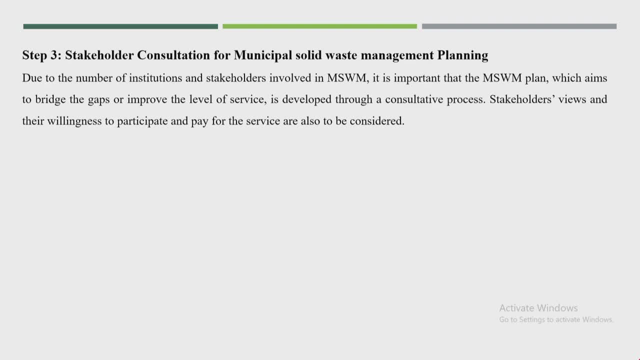 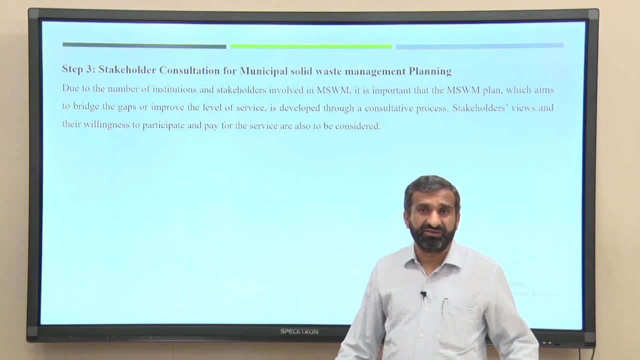 particular gaps, like gaps could be like: we do not have treatment facility, we do not have sanitary landfill is available under the current situation is saying that the waste is highly biological in nature, could produce Good quality of product Through composting or biological treatment facility. under and also we required the special 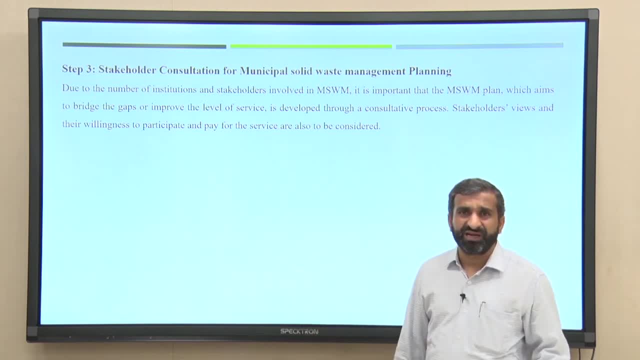 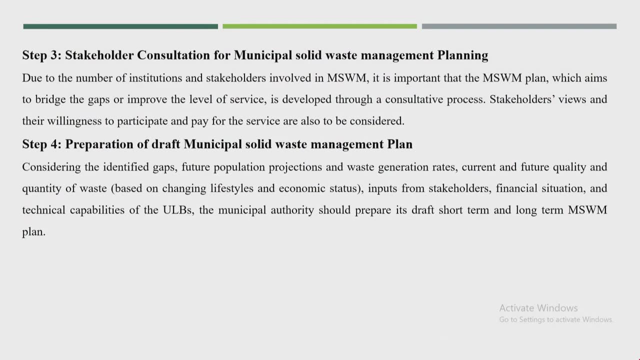 facility for the sanitary landfill. likewise, we can share with the stakeholders and have discussion with them, And once the discussion is over then we can come up with draft municipal solid waste management plan, draft plan by by sitting with all technical people in the corporations or with the some. 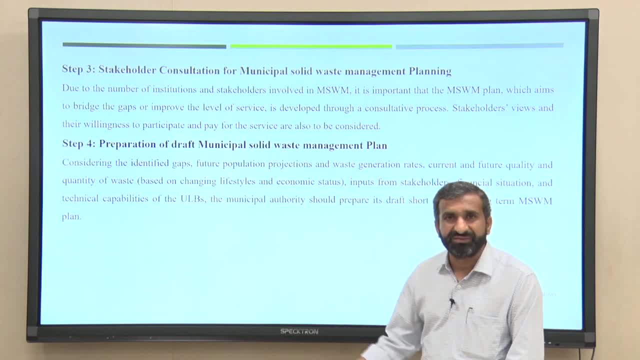 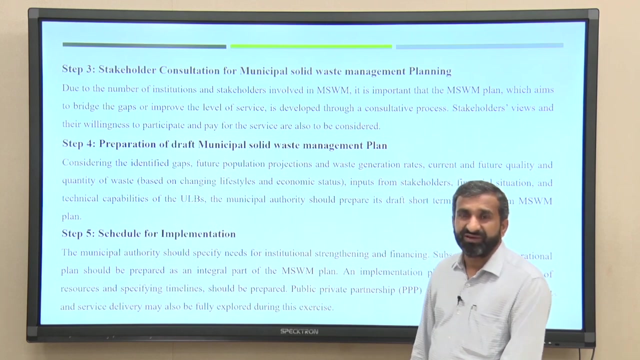 some Outside academicians or or some researcher can by by participation, participation of participations of the researcher also could possible into the while in the preparation of draft proposal. then create the schedule for implementation, because the timeline, financial viability, manpower requirement, that has to be discussed. 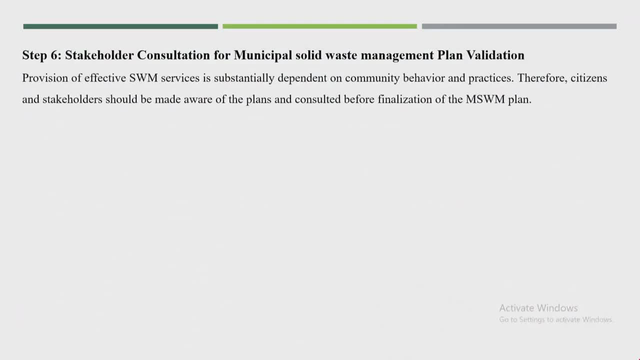 And then, Then, And then, once it is over, then again you go to the same stakeholder consultation and share them. this is what has been the thought come up into the proposal, like the, the discussion, the, the point I was discussing about. when you are planning for incision facility, you 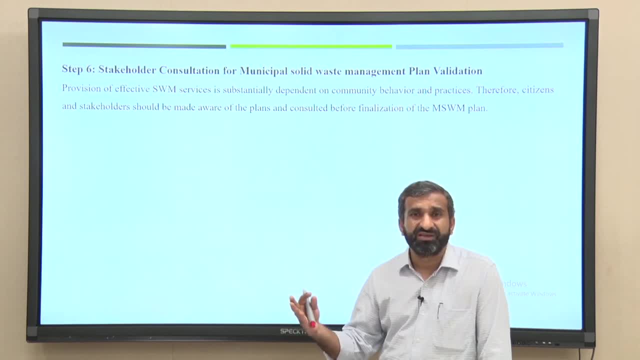 need to also look upon and need to talk about the stakeholders. if they will start some incision facility, So the all recyclable matters, They would not be able to collect it so so maybe they can oppose also and suppose they will. they will oppose or do not find much beneficial. again we will go to the go back. 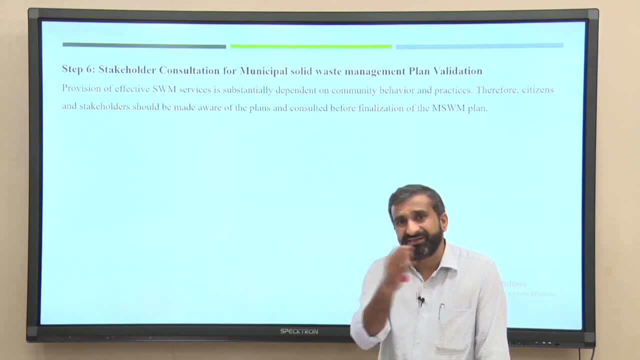 to the draft proposal preparation. so likewise we can go again and again, and again having the stakeholder. that is why, see the step 3 and step 6 is specially given for the stakeholder discussions, So that every time, whatever the proposal you come up, you have discussion with the stakeholder. 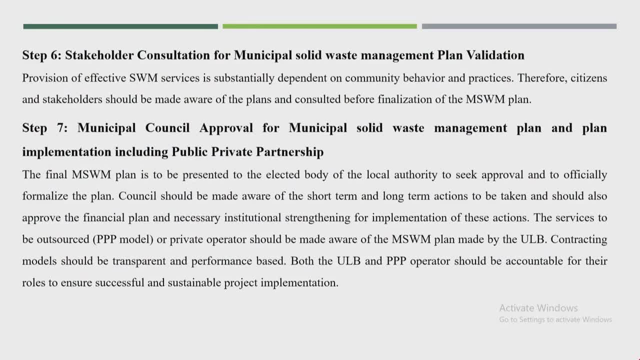 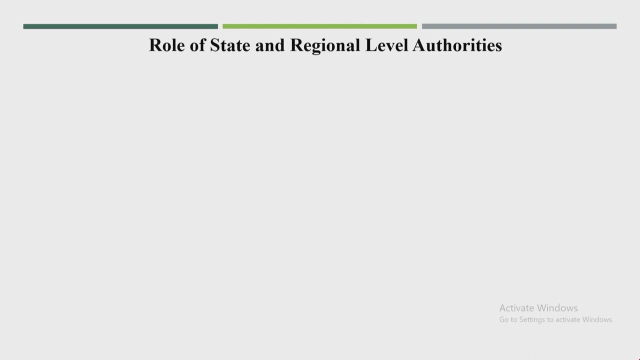 and finally, once the the stakeholders is accepted- all the points or whatever the proposal has been created by the local authority- then finally it will go to the municipal council approval for solid waste management of plan plan. Okay, Okay, Okay, Okay And finally this plan will be accepted and will be implemented. so this is the best way. 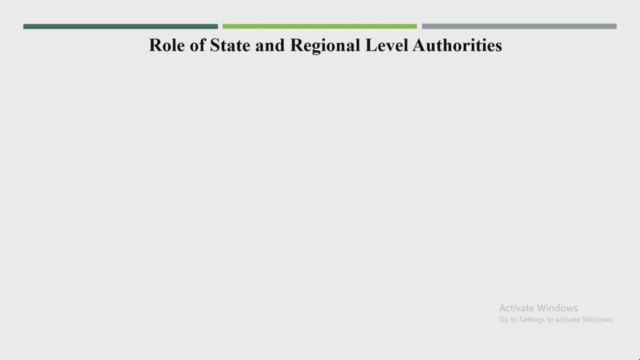 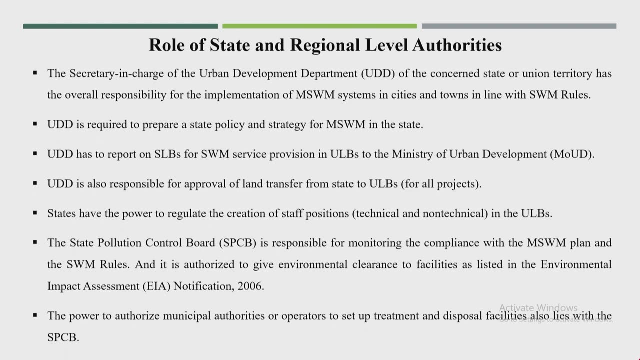 to prepare the solid waste management plan. and now the role of state and regional level authority like secretary in charge of the urban development department of the concern state or union territory has the overall responsibility for the implementation of MSWM system in the cities and town in the line of SWM rule, and this same urban development department is 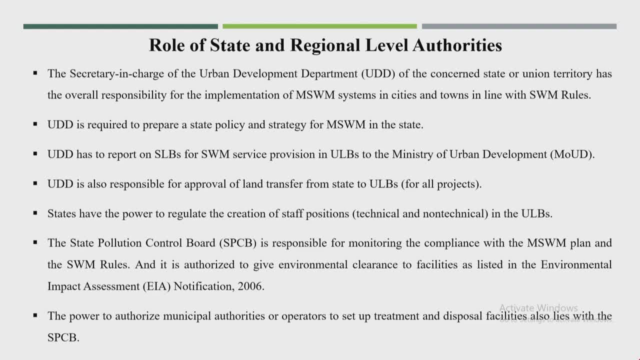 required to prepare a state policy strategy for MSWM plan and same urban development department has to report to the state bodies for SWM service provision and ELB to them, to the ministry of urban development. and same UDD is also responsible for approval of land transfer. 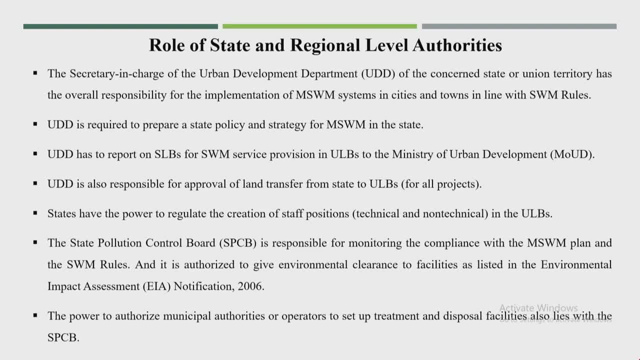 from the state to ELB. states have have the power to regulate the creation of staff position, like technical, non-technical, and also also the very important role by state position control board is responsible for monitoring the compliance with the SWM plan and SWM rule. it is authorized to give environmental clearance to facilitate the listed in the environmental 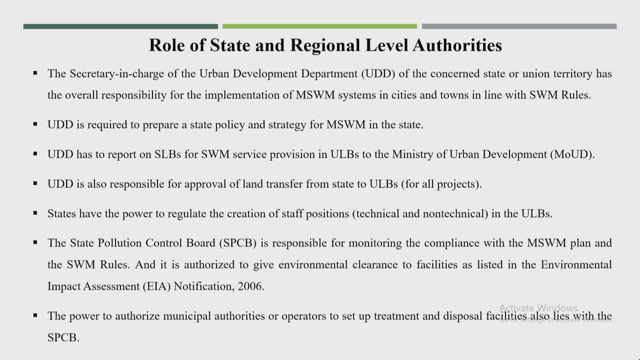 impact assessment notification 2006.. Okay, And the power to authorize municipal authority or operators to set up a treatment disposal facility also lies with the state pollution control board. So I think this is a very important role by state and regional level authorities, like specially the urban development department. so the secretary is playing the major role. 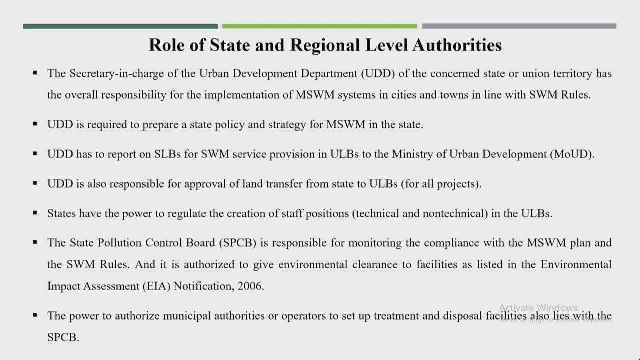 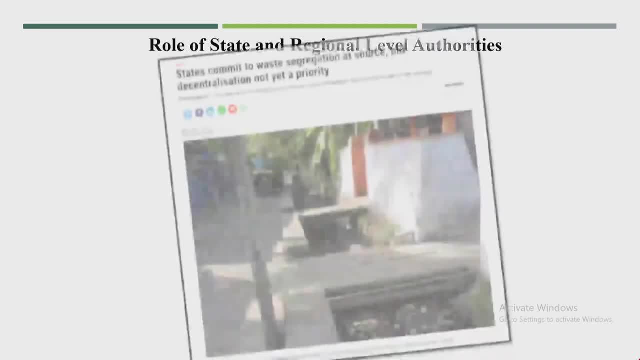 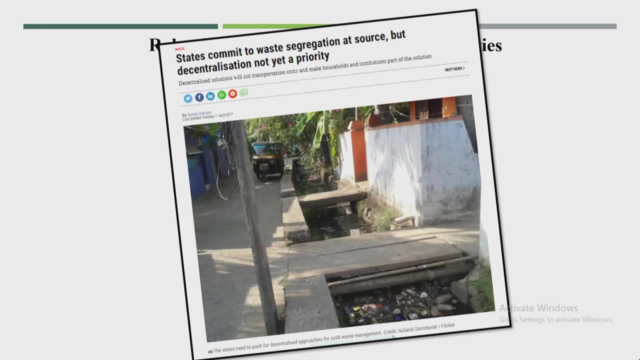 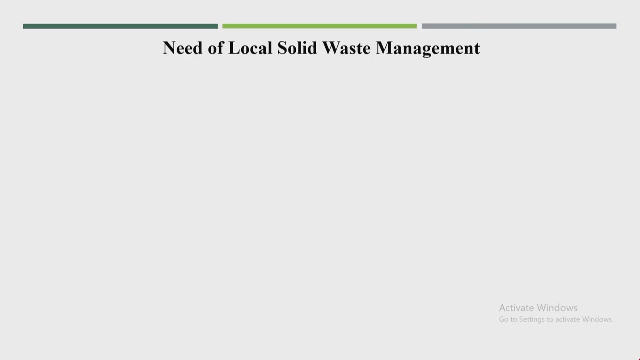 here and after that. for implementation, ULB is the important one and for monitoring, state pollution control board is important, important stakeholders. So this is one news: that state commit to waste segregation at source but decentralize and not it at a priority. this was one news. 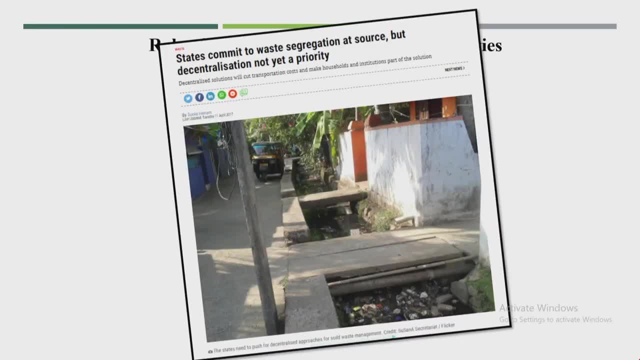 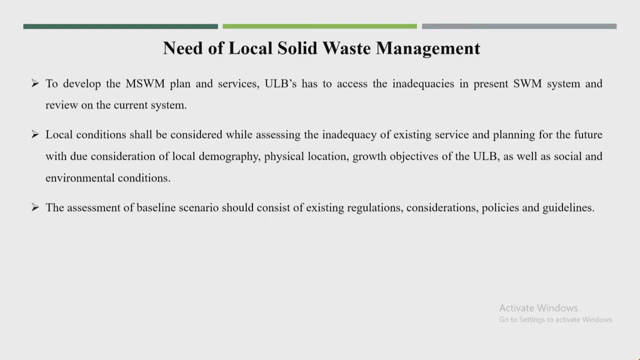 So why? because the we have map plan, we have a lot of ideas, but still such kind of news news are coming. Why Because there is a need of local solid waste management plan To develop a MSW plan, a service ULB has to assess the inadequacy to in in present SWM. 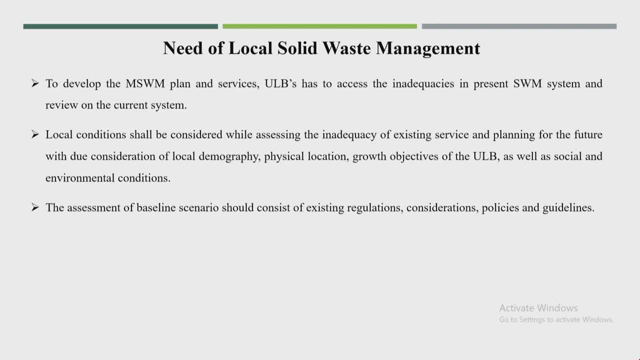 system and review the current system. So local condition shall be considered while assessing the inadequacy of existing services and the the. the idea is a local. what do you? what is the meaning of local solid waste management? Why? Because there is a need of local solid waste management plan. 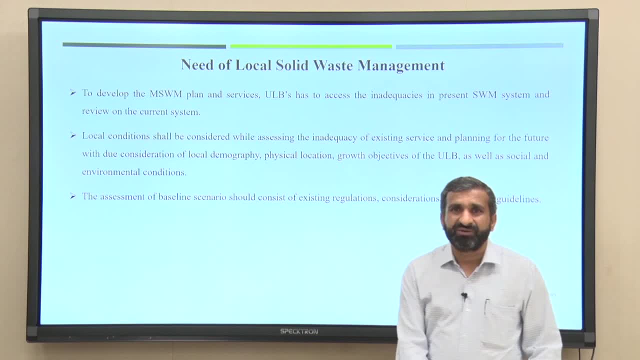 So it is again depend upon the local conditions. I would not say it is a climatic condition, local geological or climatic condition like, take example, of northeast part of India where rain is more than 6 months, somewhere 8 months rain in a year, or hilly conditions in specially. 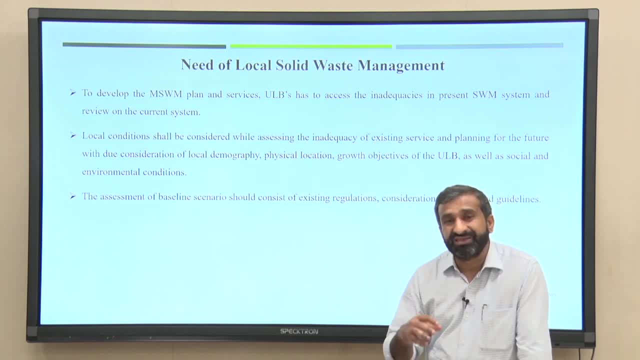 in Meghalaya or Arunachal Pradesh. So it is a local geological or climatic conditions. So it is again depend upon the local conditions. I would not say it is a climatic condition. So in that case now, whether the whatever, the whatever, the priorities in the other part, 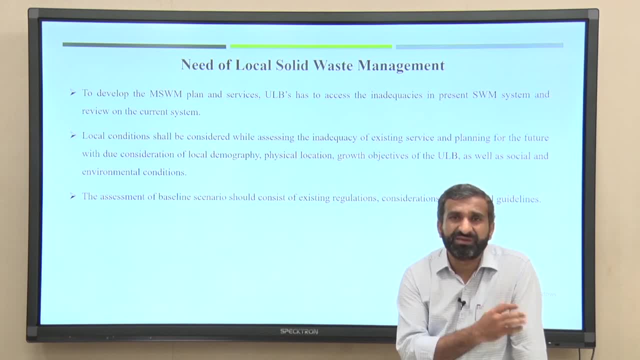 of India in the plain areas, like they can have the very big, big sanitary landfill, they can have very big composting facility in the open areas could be possible. So is it possible to do it in these kind of areas? No local condition says the 8 months rain means you cannot have the landfill is very 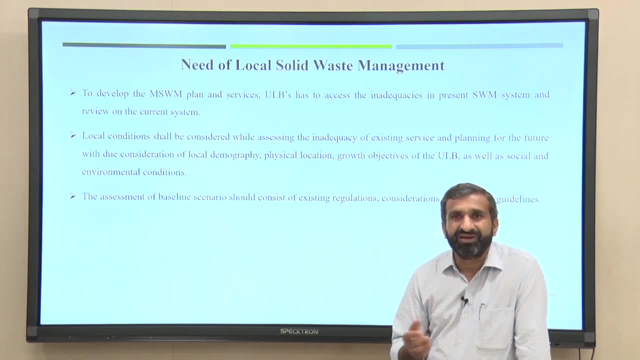 difficult. The ground water table will be very high So it is very difficult to have the have the sanitary landfills in such areas. even the sanitary landfills, the type of sanitary landfills, will be different in the hilly regions. We cannot go for simple excavation or area methods. we have to go for depression kind. 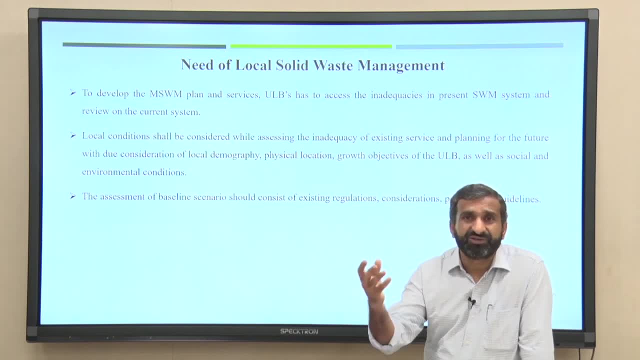 of landfills in the in the but, but there also, if you have the landfill in the hilly areas, there are a lot of leachate productions And a lot of production. Yeah, A lot of pollution will come up in the. both the cases the local condition says that need. 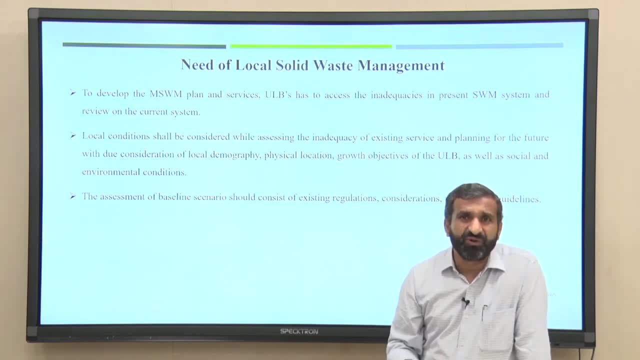 to have more treatment facility should be provided. So rather than looking on to the other states in the other part of India, they need not to have the similar kind of facilities. So here here specially, will be required more info. house to house collections, Yeah. 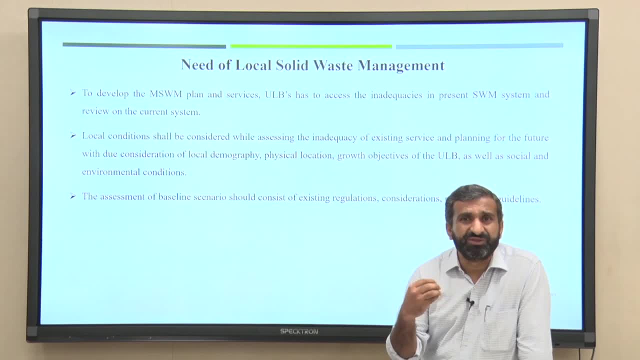 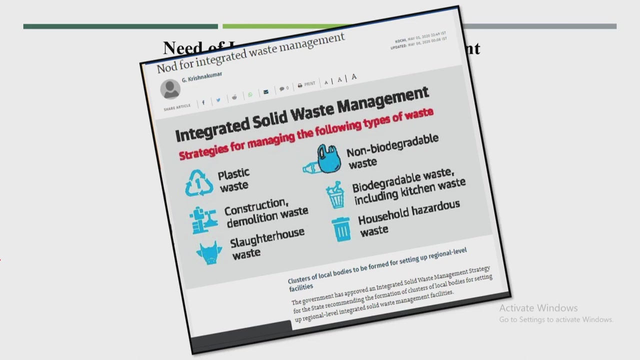 Yeah, So the waste to house collection system is very important. segregated way under treatment is more priority rather than the landfilling. I think that is what the local solid waste management plans also need to be discussed. So this is solid waste management strategies for managing the following type of waste like: 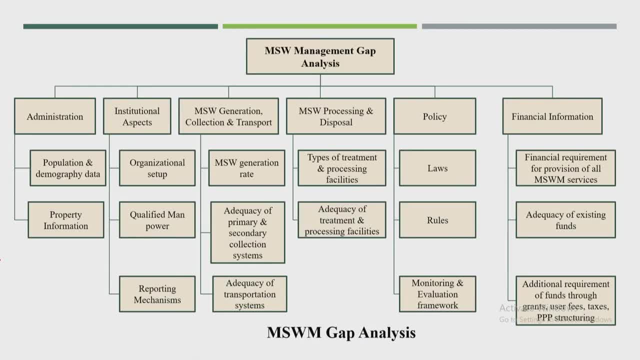 this one news. This is the gap analysis of solid waste management- Yeah, of solid waste management. So when you are checking up any, or when you are going through the any reports of solid waste management plan, so try to go through these particular gap analysis and see that. 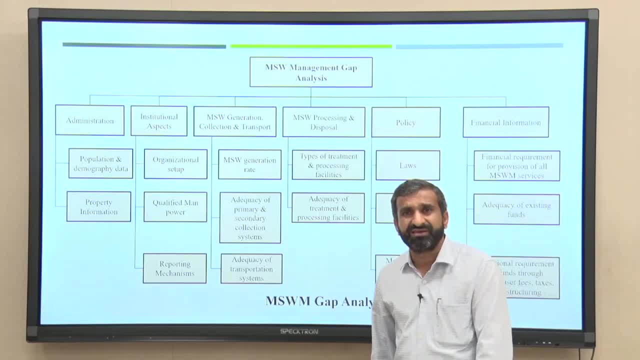 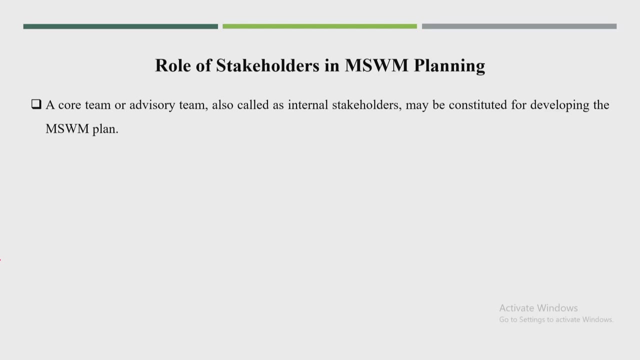 whether such kind of project or such kind of plans are prepared based on the proper technical and non-technical understanding. So now is the role of stack holders in the MSWM, MSWM planning. A core team or advisory team, also called as internal stack holder, may be constitutes for 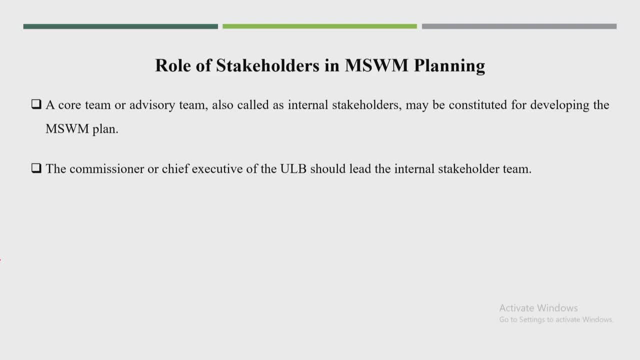 developing the MSWM plan. The commissioner or chief executive of the ULB should lead the internal stack holder team And typical stack holders for MSWM system includes household business management business, businesses, industry, informal sectors, local government, NGOs, CBOs, self. 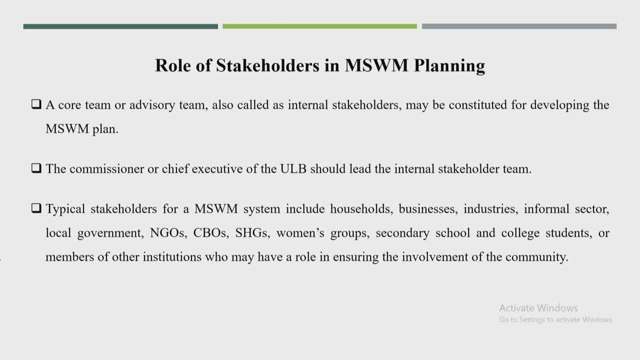 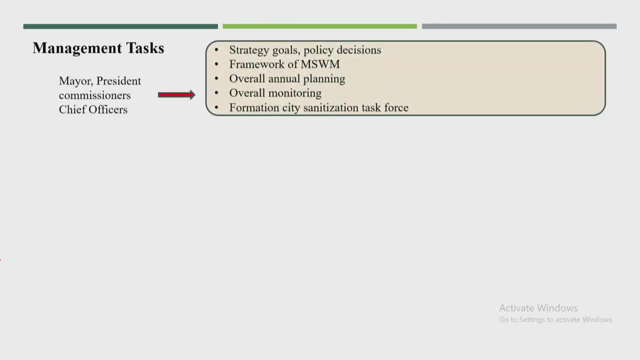 help group, women's group, secondary school, college students or other member of the institutes may play major role. Now the management task. like in the any ULBs, you will have the. the boss of the corporation is a mayor or president Or commissioners or chief officers. 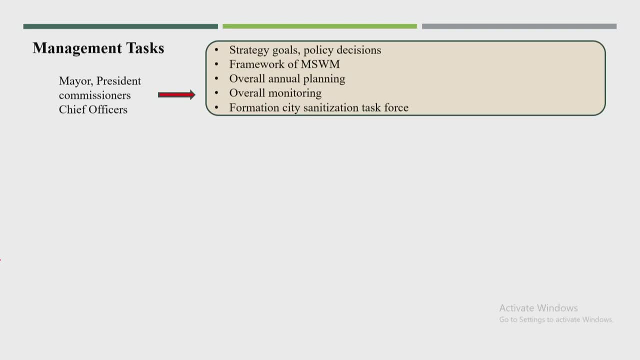 Their task will be to strategy, goal policy, decision frame, working, overall annual planning, overall monitoring, like, say, health officers or engineers or for the technical supervision guidance operation, quality control operation, supervision, stack holder, management, responsibility of the service contracts. they have to be look upon by the health officers and engineers. 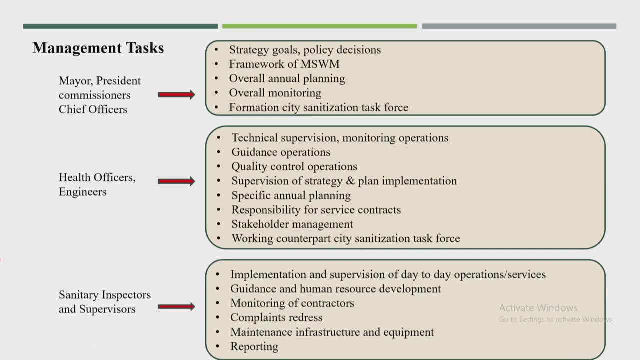 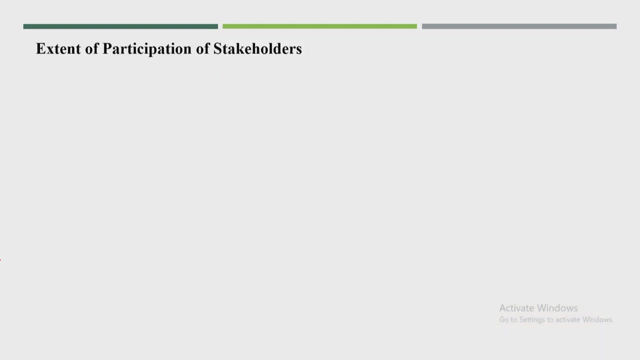 And finally, sanitary inspectors and supervisor. they have to look for implementation and supervision of day to day operation, guidance in human resources, monitoring of contracts- complaint should be re-addressed- and maintenance infrastructure equipment. that has to be look from the sanitary inspectors and supervisor. 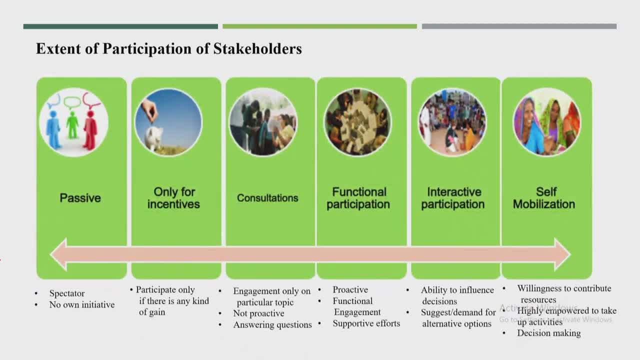 Now what extent the participation of stack holders should be considered. Okay, stockholders could be possible. So I think if you talked about the, the passive one, passive means their own. they would not get any initiatives and self mobilization. they have the very good. 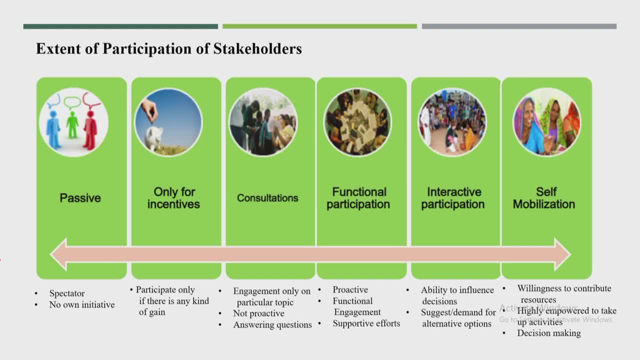 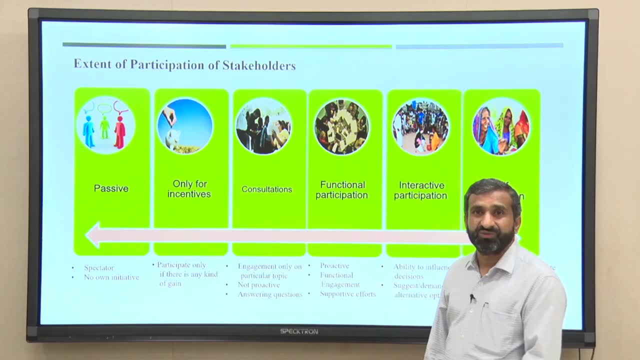 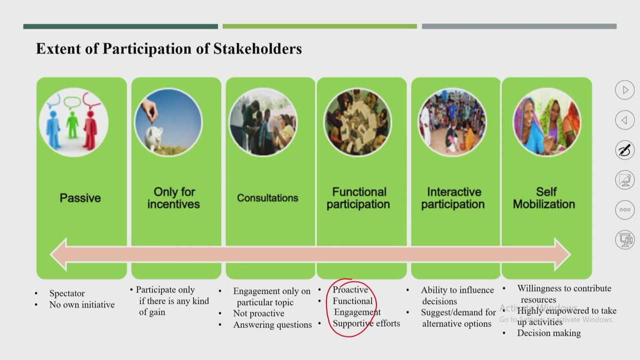 willingness. So there, I think, based on this, we can see that what kind of extension or engagement of stakeholders could be possible. So maybe I think here, major one is a proactive, functional engagement. This is also need to be see, that we need not to accept only those. 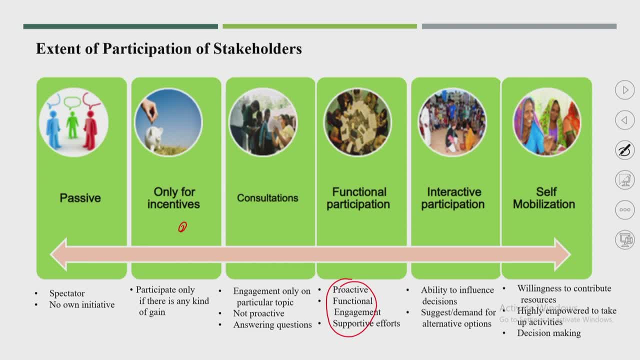 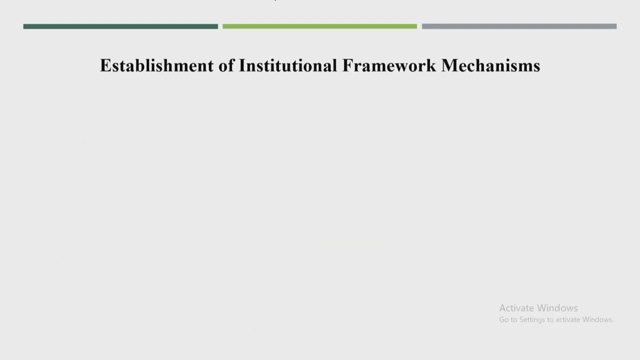 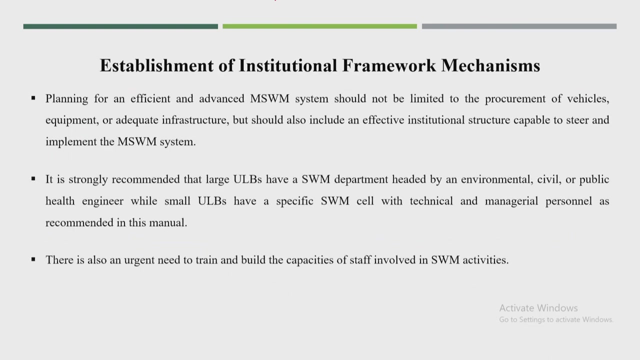 are required are coming into the incentive for the only the for purpose of incentives, but also see that how best they will be, they are the beneficial for us, Okay. And also the interactive participation. this is also good, acceptable for such kind of people, Okay. Now the establishments of institutional framework mechanism. So is a planning for?